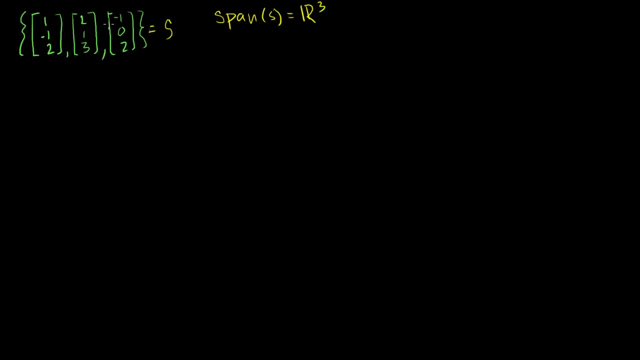 And it seems like it might be, If each of these add new information. it seems like maybe I could describe any vector in r3 by these three vectors, by some combination of these three vectors. And the second question I'm going to ask is: are they? 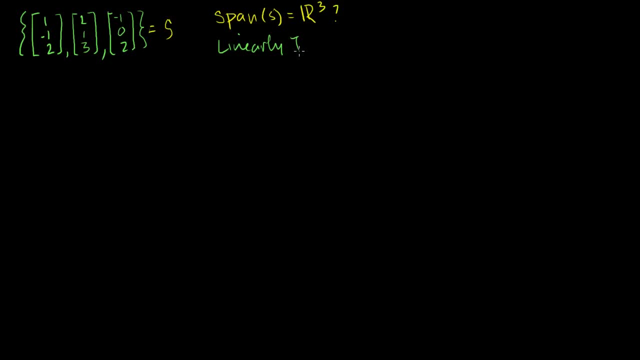 linearly independent And maybe I'll be able to answer them at the same time. So let's answer the first one. Do they span r3?? And to span r3, that means some linear combination of these three vectors should be able to construct. 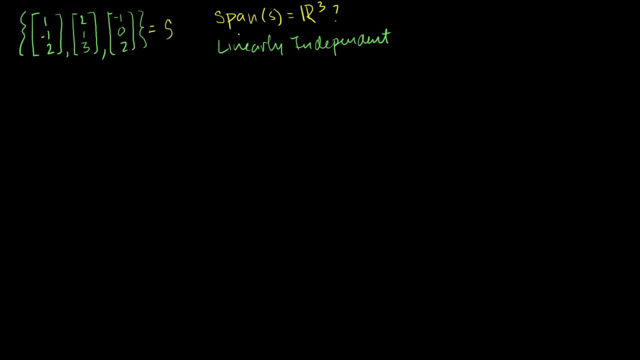 any vector in r3.. So let me give you a linear combination of these vectors So I could have c1 times the first vector, 1 minus 1, 2, plus some other arbitrary constant, c2, some scalar times the second vector. 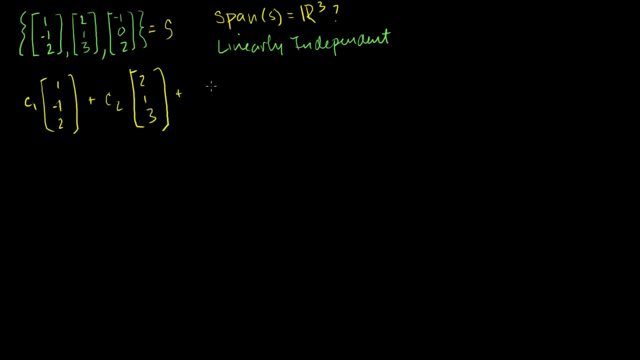 2., 1., 3. Plus some third scaling factor times the third vector minus 1,, 0,, 2.. I should be able to, using some arbitrary constants, take a combination of these vectors that sum up to any vector in. 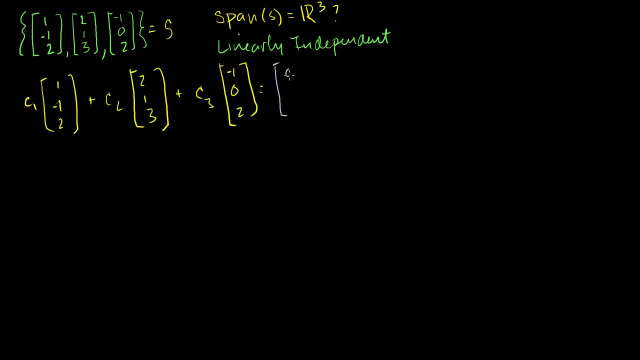 r3, and I'm going to represent any vector in r3 by the vector a, b and c, where a, b and c are any real numbers. So this, if I can, if you give me any a, b and c and I can give you a formula for telling you. 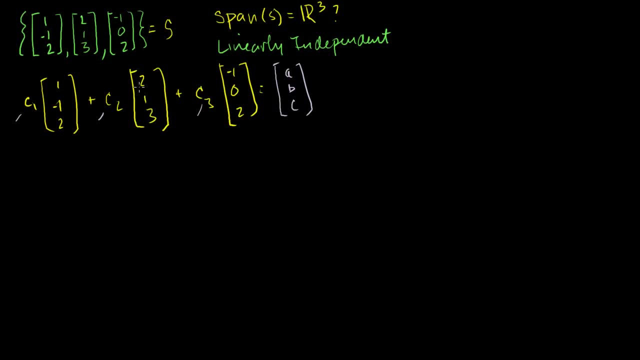 what your c3's, your c2's and your c1's are, then that essentially means that it spans r3. Because if you give me a vector, I can always tell you how to construct that vector with these three. So let's see if I can do that. 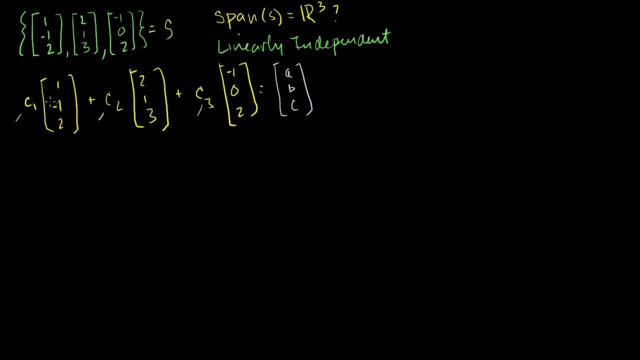 So just from our definition of scalar multiplication of a vector, we know that c1 times this vector. I could rewrite it if I want, And I normally skip this step, but I really want to make it clear. So c1 times this, I could just rewrite it as 1 times c, it's. 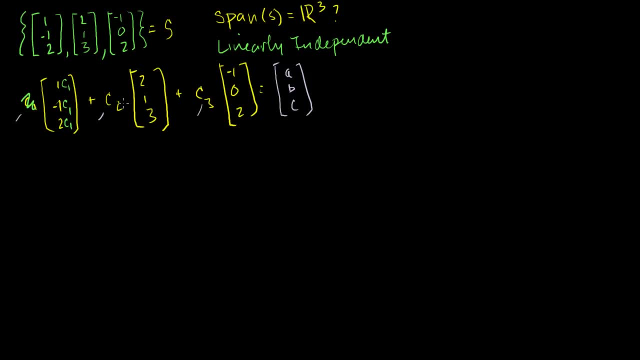 each of the terms times c1.. Similarly, c2 times, this is the same thing as each of the terms times c2.. And c3 times, this is the same thing as each of the terms times c3.. I want to show you that everything we do, it just. 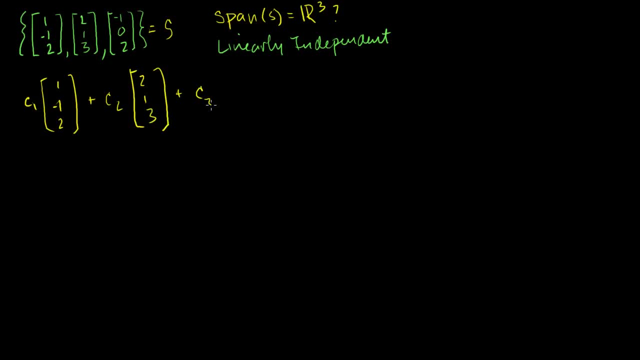 Plus some third scaling factor times, the third vector minus 1,, 0,, 2.. I should be able to, using some arbitrary constants, take a combination of these vectors that sum up to any vector in r3. And I'm going to represent any vector in r3 by the vector a. 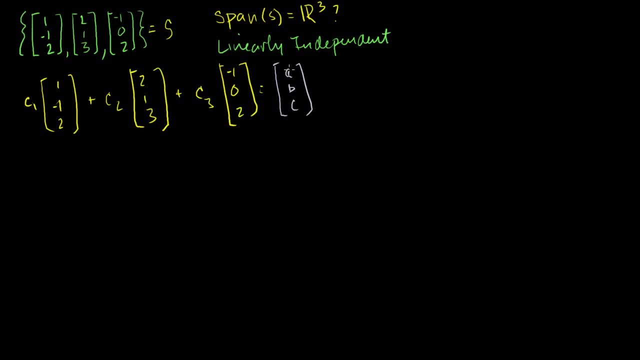 b and c, where a, b and c are any real numbers. So this, if I can, if you give me any a, b and c, I'm going to give you a formula for telling you what your c3's, your c2's. 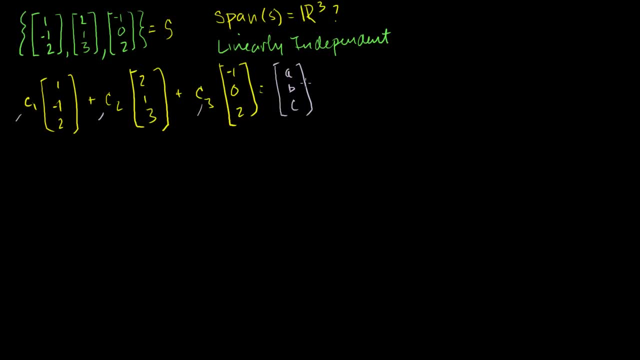 and your c1's are, then that essentially means that it spans r3. Because if you give me a vector, I can always tell you how to construct that vector with these three. So let's see if I can do that. So just from our definition of scalar multiplication of a, 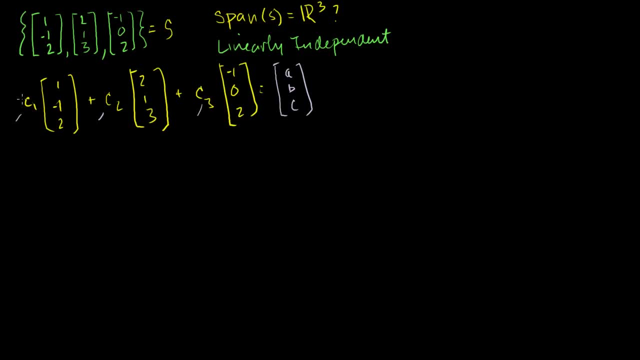 vector. we know that c1 times this vector. I could rewrite it if I want, And I normally skip this step, but I really want to make it clear. So c1 times this, I could just rewrite it as 1 times c it's. 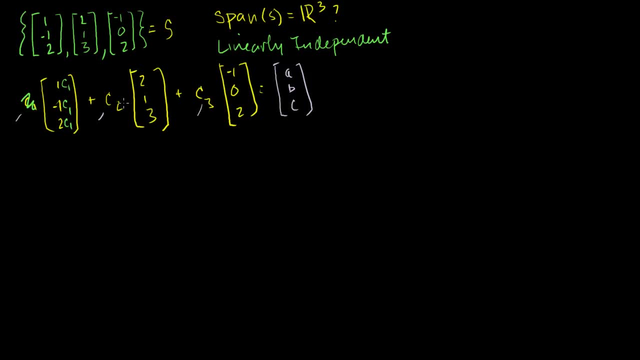 each of the terms times c1.. Similarly, c2 times, this is the same thing as each of the terms times c2.. And c3 times, this is the same thing as each of the terms times c3.. I want to show you that everything we do, it just. 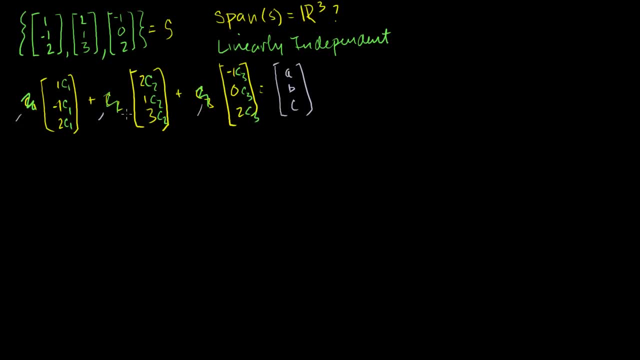 formally comes from our definition of vector, of multiplication of a vector times a scalar, which is what we just did, or vector addition, which is what we're about to do. So vector addition tells us that this term plus this term plus this term needs to equal that term. 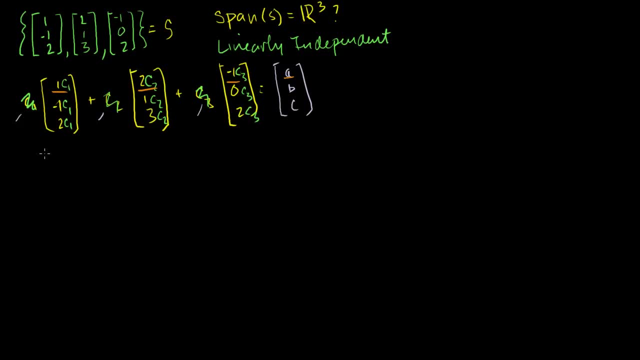 So let me write that down. We get c1 plus 2c2. minus c3 will be equal to a. Likewise we can do the same thing with the next row. Minus c1 plus c2 plus 0c3 must be equal to b. 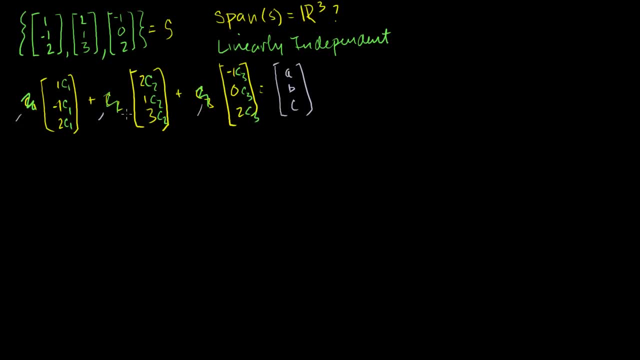 formally comes from our definition of multiplication of a vector times a scalar, which is what we just did, or vector addition, which is what we're about to do. So vector addition tells us that this term plus this term plus this term needs to equal that term. 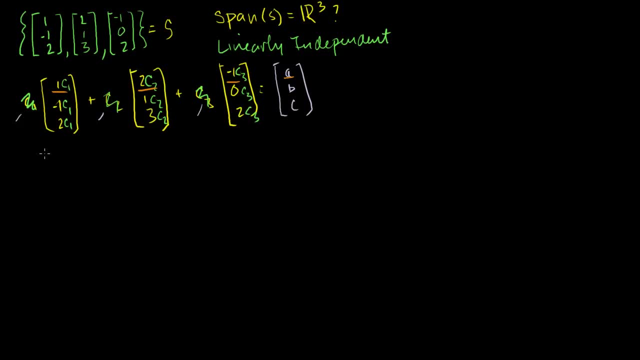 So let me write that down. We get c1 plus 2c2. minus c3 will be equal to a. Likewise we can do the same thing with the next row. Minus c1 plus c2 plus 0c3 must be equal to b. 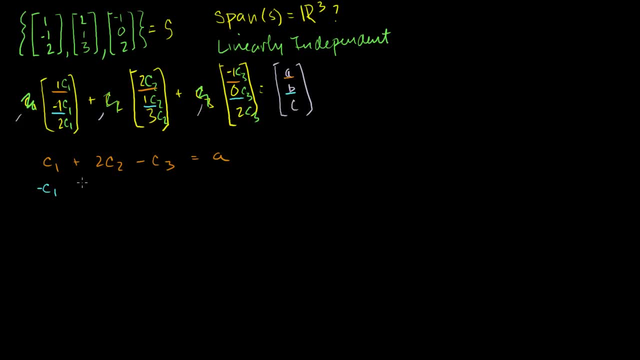 So we get minus c1 plus c2 plus 0c3, so we only have to write: that is going to be equal to a, b, And then finally, let's just do that last row: 2c1 plus 3c2 plus 2c3 is going to be equal to c, right there. 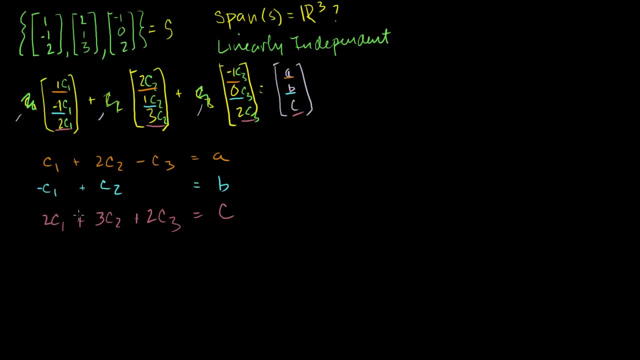 Now let's see if we can solve for our different constants. So I'm going to do it by elimination. I think you might be familiar with this process. I think I've done it in some of the earlier linear algebra videos Before I started doing this. 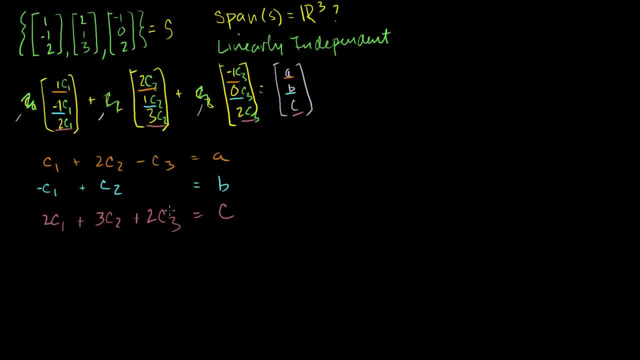 I started doing a formal presentation of it And I'm going to review it again in a few videos from now. But I think you understand how to solve it this way. What I'm going to do is I'm going to first eliminate these two terms and then I'm going to eliminate this term. 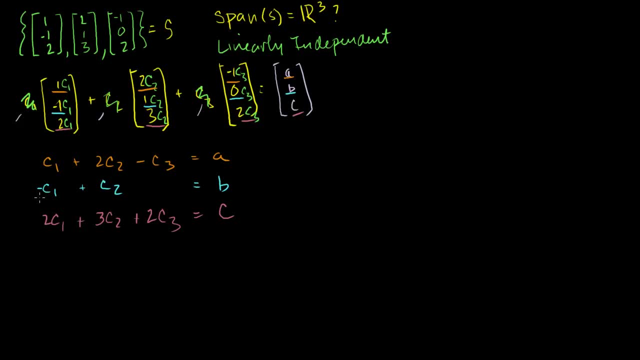 And then I can solve for my various constants. So if I want to eliminate this term right here, what I could do is I could add this equation to that equation Or, even better, I can replace this equation with the sum of these two equations. 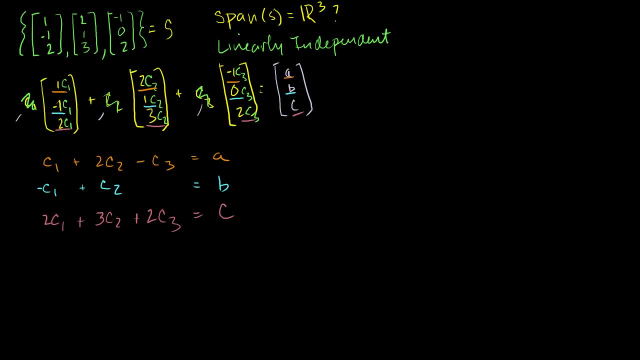 So let me do that. So I'm just going to add these two equations. OK, OK, OK. So I'm going to add these two equations to each other and replace this one with that sum. So minus c1, plus c1.. 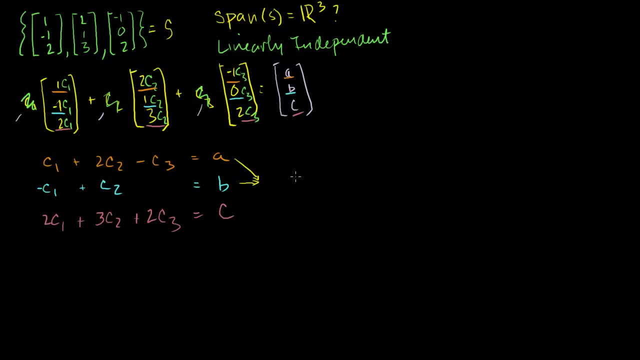 That just gives you 0. I can ignore it. Then c2 plus 2c2.. That's 3c2.. And then 0 plus minus c3 is equal to minus c3. And I'm replacing this with the sum of these two. 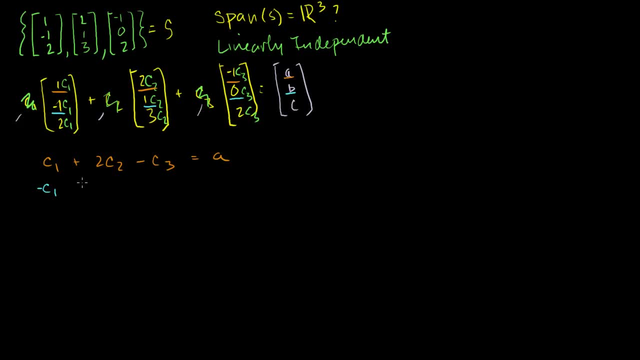 So we get minus c1 plus c2 plus 0c3, so we only have to write: that is going to be equal to b. And then, finally, let's just do that last row: 2c1 plus 3c2 plus 2c3 is going to be equal to c, right there? 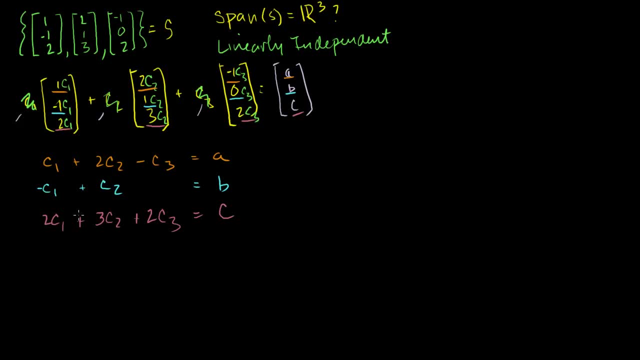 Now let's see if we can solve for our different constants. So I'm going to do it by elimination. I think you might be familiar with this process. I think I've done it in some of the earlier linear algebra videos before I started doing a. 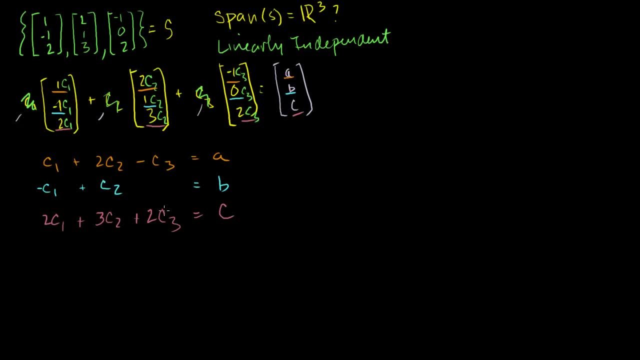 formal presentation of it, And I'm going to review it again in a few videos from now, But I think you understand how to solve it this way. What I'm going to do is I'm going to first eliminate these two terms and then I'm going to eliminate this term and 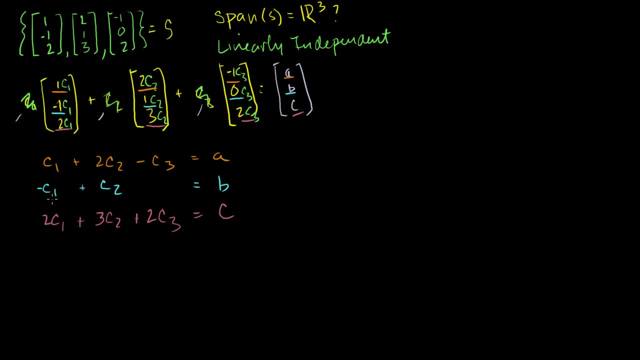 then I can solve for my various constants. So if I want to eliminate this term right here, what I could do is I could add this equation to that equation Or, even better, I can replace this equation with the sum of these two equations. 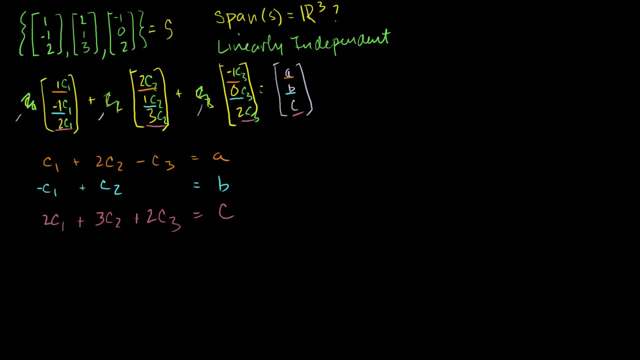 So let me do that. So I'm just going to add these two equations to each other and replace this one with that sum. So minus c1 plus c1, that just gives you 0. I can ignore it. Then c2 plus 2c2, that's 3c2.. 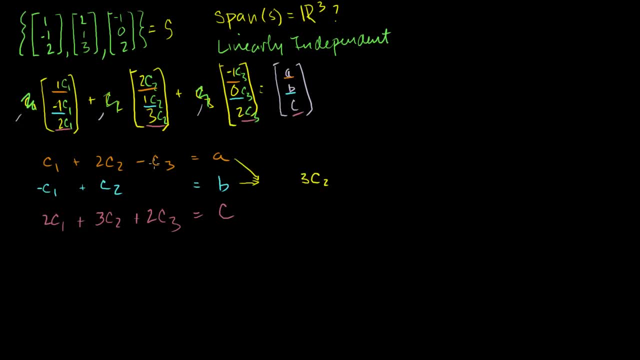 And then 0 plus minus c3 is equal to minus c3. And I'm replacing this with the sum of these two. So b plus a equals b plus a. Let me write down that first equation on the top. So the first equation: 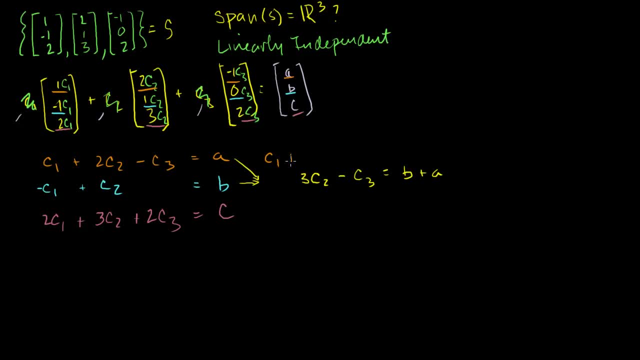 I'm not doing anything to it. So I get: c1 plus 2c2 minus c3 is equal to a. Now, in this last equation I want to eliminate this term, So let's take this equation and subtract from it 2 times. 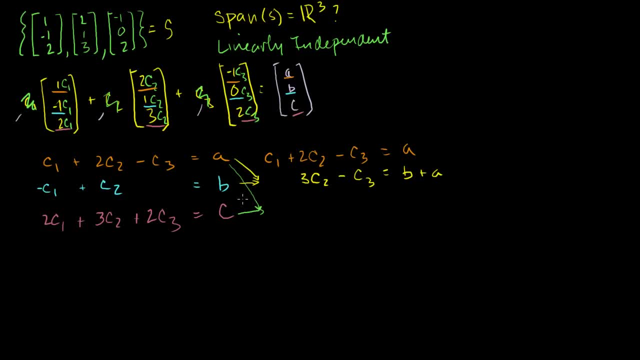 this top equation, So you could also view it as: let's add this to minus 2 times this top equation. And since we're almost done using this- we actually even wrote it- Let's just multiply this times minus 2.. So this becomes a minus 2c1, minus 4c2, plus 2c3. 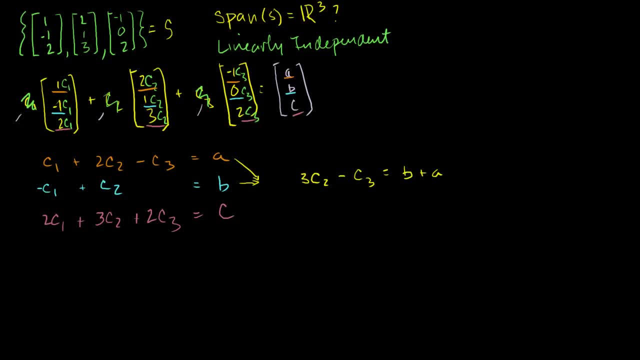 So b plus a equals b plus a. Let me write down that first equation on the top. So the first equation, I'm not doing anything to it. So I get: c1 plus 2c2 minus c3 is equal to a. 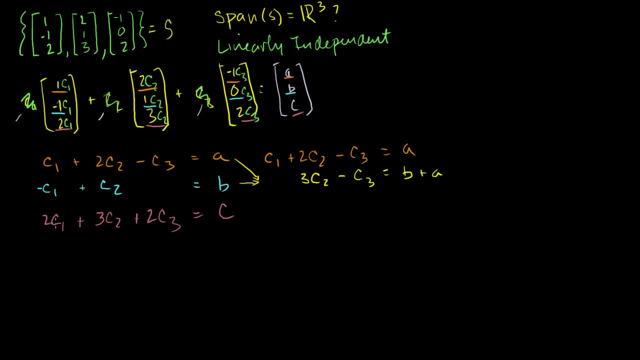 Now, in this last equation, I want to eliminate this term. So let's take this equation and subtract from it 2 times this top equation, So you could also view it as: let's add this to minus 2 times this top equation. And since we're almost done, 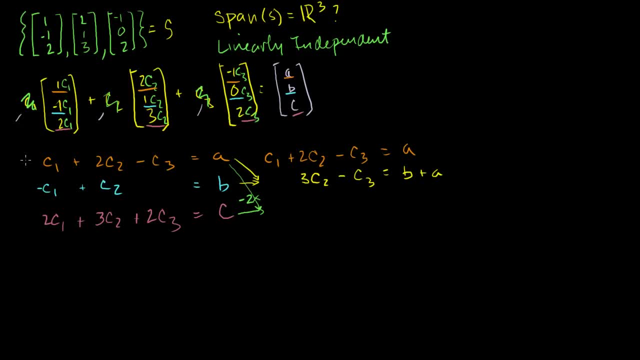 using this. we actually even wrote it. Let's just multiply this times minus 2.. So this becomes a minus 2c1 minus 4c2 plus 2c3.. So plus 2 plus 2c3 is equal to minus 2a, right. 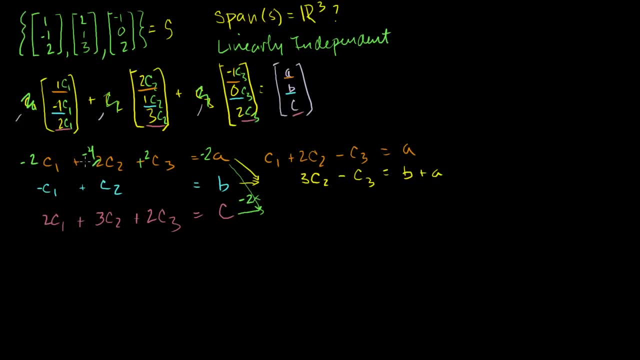 If you just multiply each of these terms- I want to be very careful, I don't want to make a careless mistake- Minus 2 times c1, minus 4, plus 2.. And then minus 2.. And now we can add these two together. 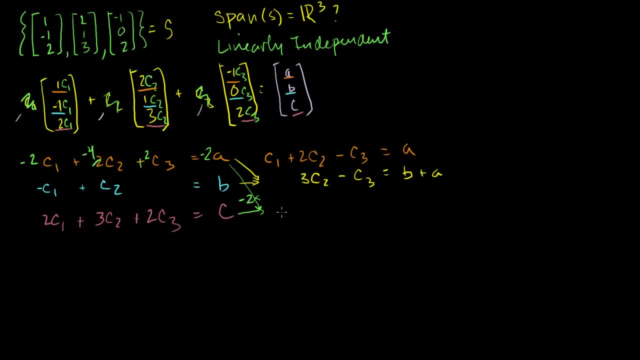 And what do we get? The 2c1 minus 2c1, that's a 0.. Don't have to write it 3c2 minus 4c2,, that's a minus c2.. And then you have your 2c3 plus another 2c3. 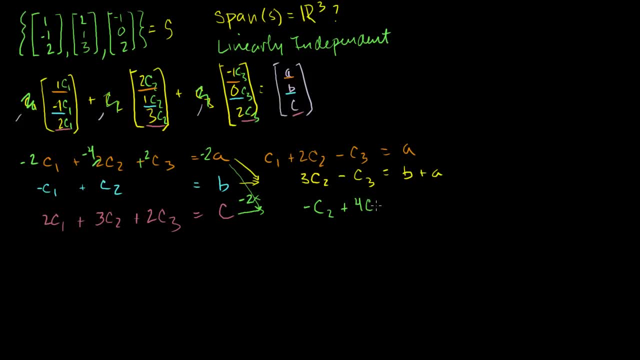 So that is equal to plus 4c3.. That's a minus c2.. That's a minus c2.. That's a minus c2.. And then you have your 2c3 plus another 2c3.. And then you have your 2c3 plus another 2c3.. 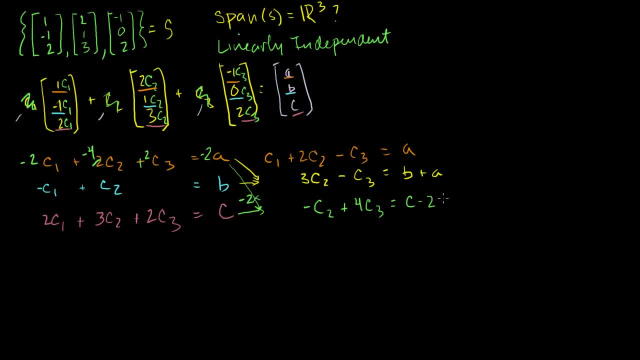 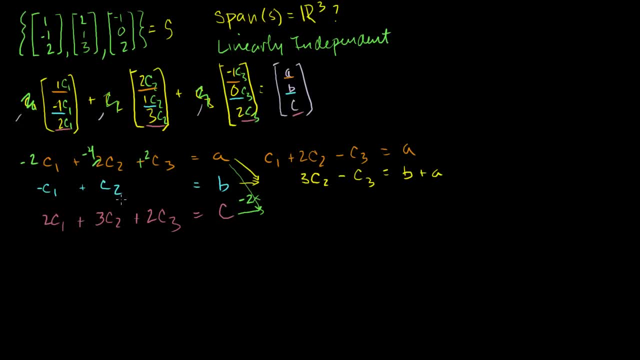 So plus 2 plus 2c3 is equal to minus 2a, right? If you just multiply each of these terms. I want to be very careful. I don't want to make a careless mistake: Minus 2 times c1, minus 4 plus 2.. 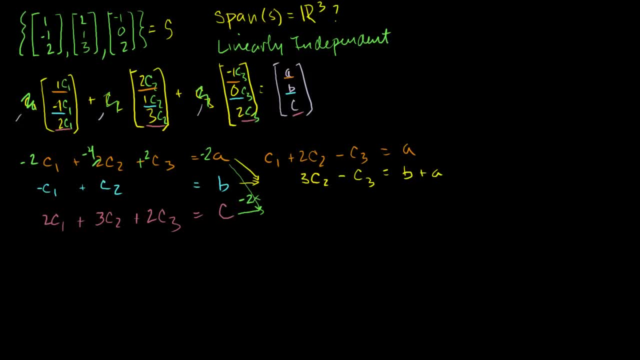 And then minus 2a, Minus 2.. And now we can add these two together And what do we get? The 2c1 minus 2c1, that's a 0. Don't have to write it. 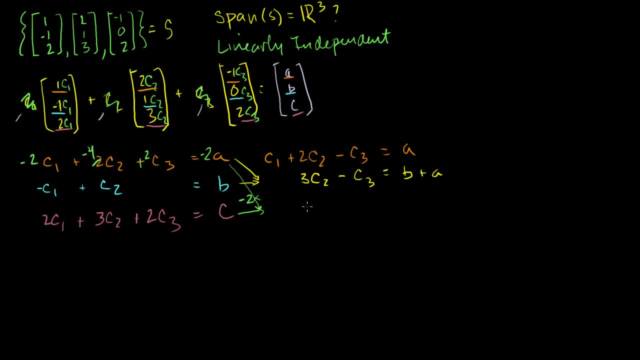 3c2 minus 4c2, that's a minus c2.. And then you have your 2c3 plus another 2c3.. So that is equal to plus 4c3, is equal to c2c3.. 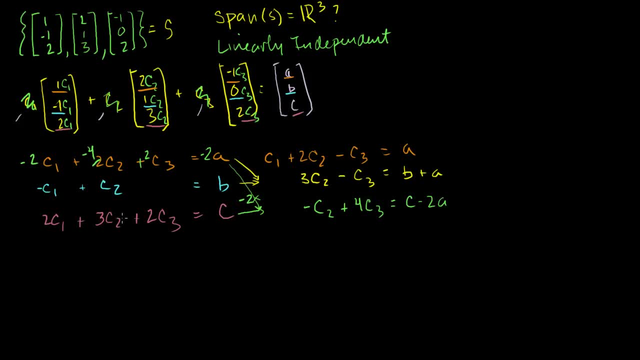 C minus 2a. All I did is I replaced this with this minus 2 times that, And I got this. Now I want to eliminate. Now I'm going to keep my top equation constant again. I'm not going to do anything to it. 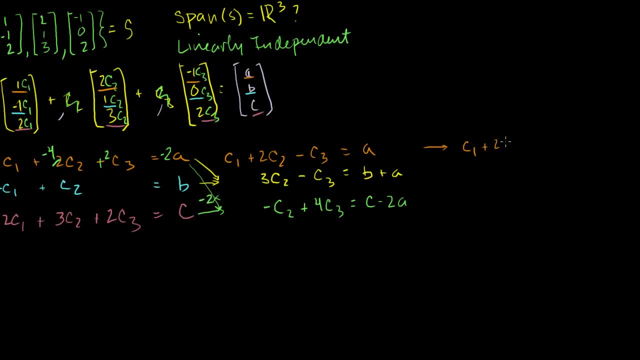 So I'm just going to move it to the right, So I get c1 plus 2c2 minus c3 is equal to a, And I'm also going to keep my second equation the same, So I get 3c2.. 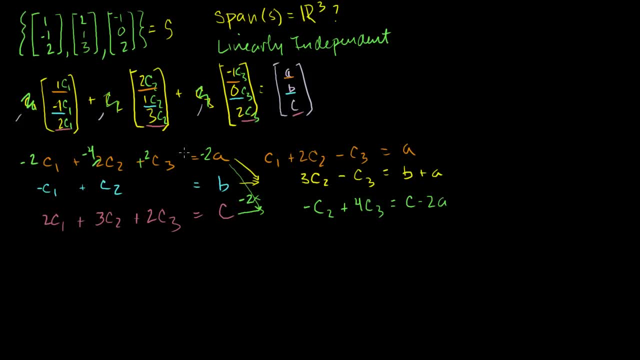 All I did is I replaced this with this minus 2 times that, And I got this. Now I want to eliminate. Now I'm going to keep my top equation constant again. I'm not going to do anything to it, So I'm just going to move it to the right. 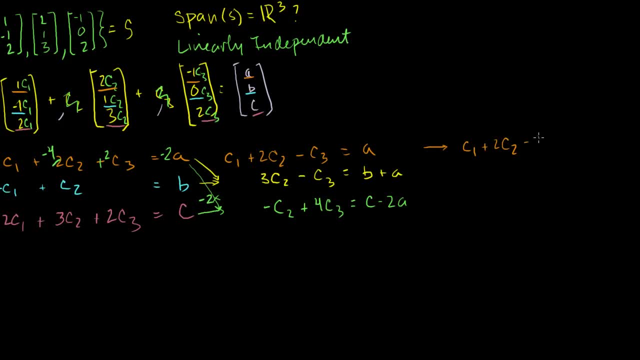 So I get c1 plus 2c2 minus c3 is equal to a, And I'm also going to keep my second equation the same, So I get 3c2 minus 2c3.. c2 minus c3 is equal to b plus a. 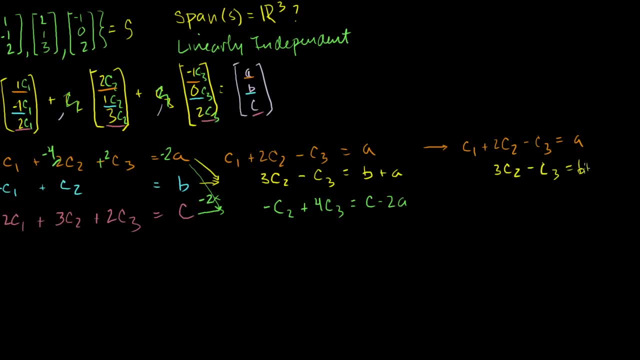 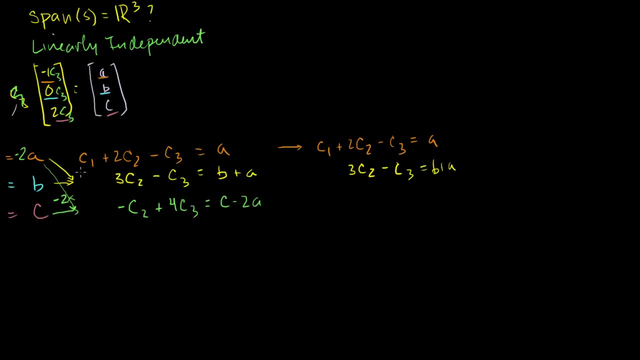 c2 minus c3 is equal to b plus a. Let me scroll over a good bit. And then this last equation I want to eliminate. My goal is to eliminate this term right here. So what I want to do is I want to multiply this bottom. 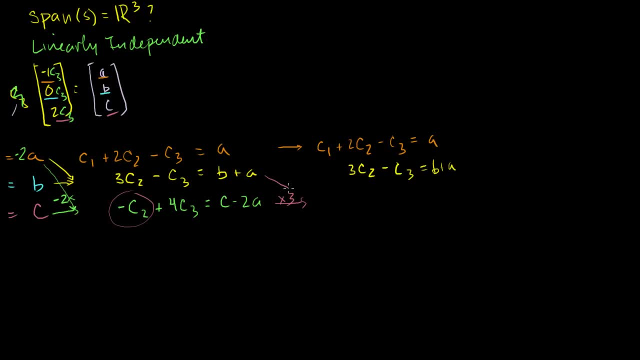 equation times 3 and add it to this middle equation to eliminate this term right here. So if I multiply this bottom equation times 3, let me just do it. Well, actually, let me, Let me make things messier. So this becomes a minus 3 plus a 3.. 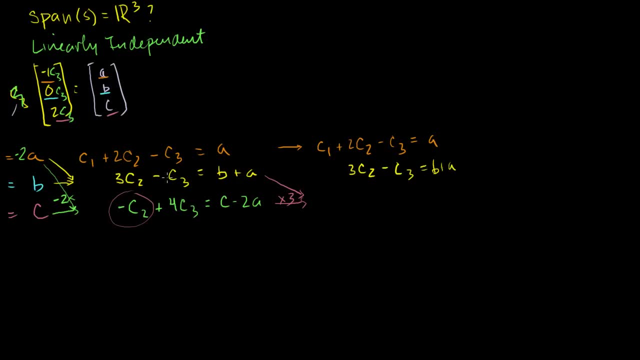 So those cancel out. This becomes a 12 minus a 1.. So this becomes 12c3 minus c3, which is 11c3.. And then this becomes a. Oh sorry, I was already done When I do 3 times this plus that those canceled out. 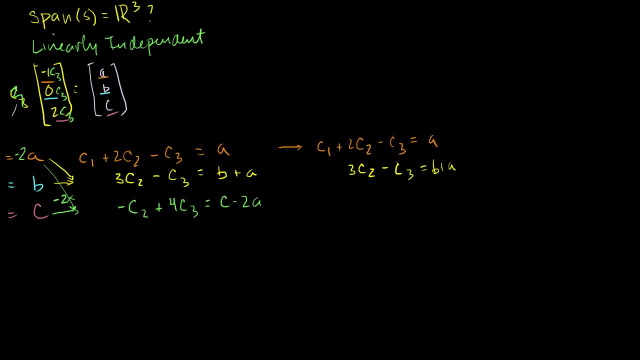 Let me scroll over a good bit. And then this last equation I want to eliminate. My goal is to eliminate this term right here. So what I want to do is I want to multiply this bottom equation times 3 and add it to this middle equation. 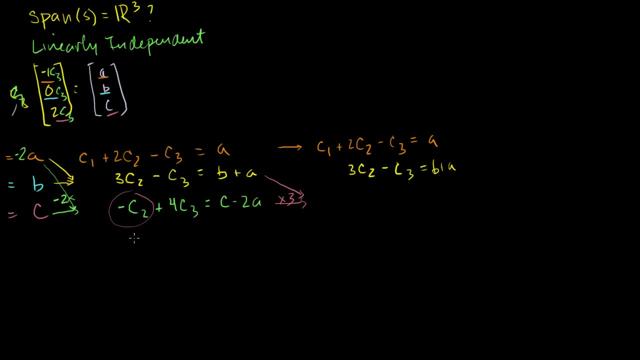 to eliminate this term right here. So if I multiply this bottom equation times 3, well, actually I don't want to make things messier- So this becomes a minus 3 plus a 3.. So those cancel out This becomes a 12 minus a 1.. 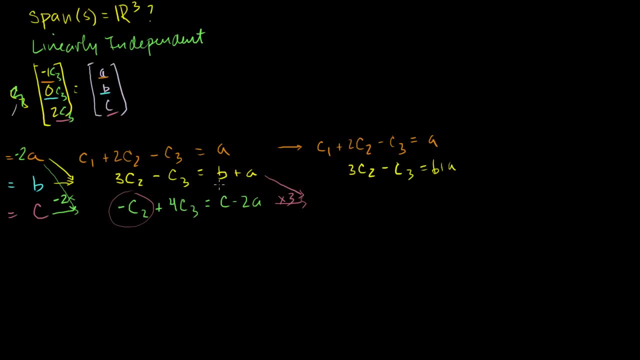 So this becomes 12c3 minus c3, which is 11c3. And then this becomes a. oh sorry, I was already done. When I do 3 times this, plus that those canceled out, And then when I multiply 3 times this, I get 12c3 minus a. 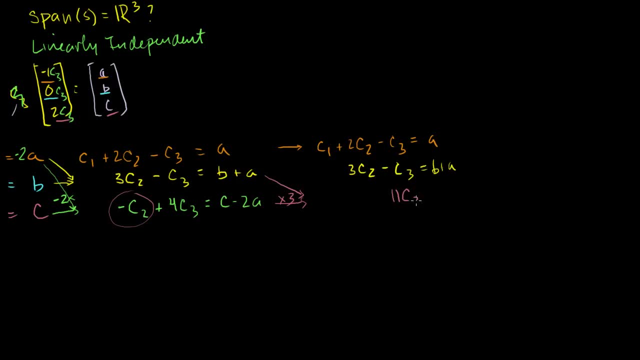 c3,, so that's 11c3.. And I multiply this times 3 plus this, So I get 3c minus 6a, right? I'm just multiplying this times 3, plus this, plus b plus a. 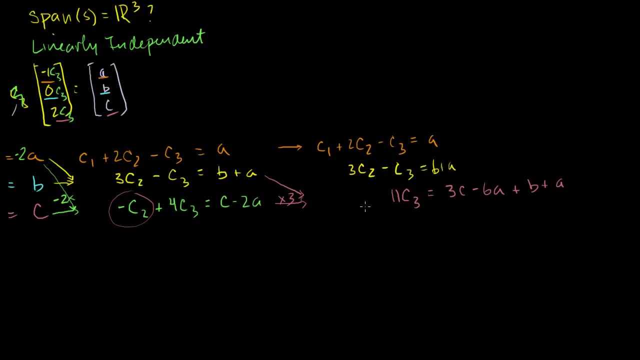 And so what can I rewrite this by? And actually I want to make something very clear. This c is different than these c1, c2s and c3s that I had up here, And I think you realize that. But I just realized that I used the letter c twice. 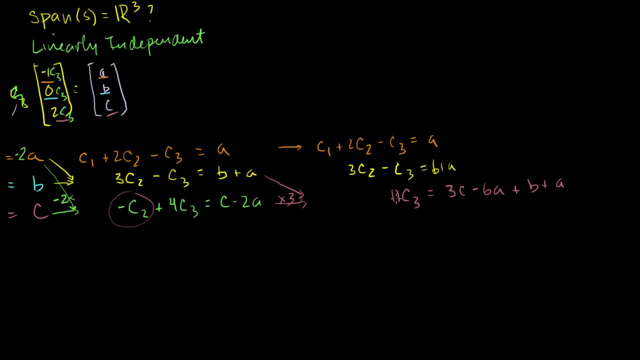 and I just didn't want any confusion here. So this c that doesn't have any subscript is a different constant than all of these things over here. So let's see if we can simplify this. So we have an a and a minus 6a. 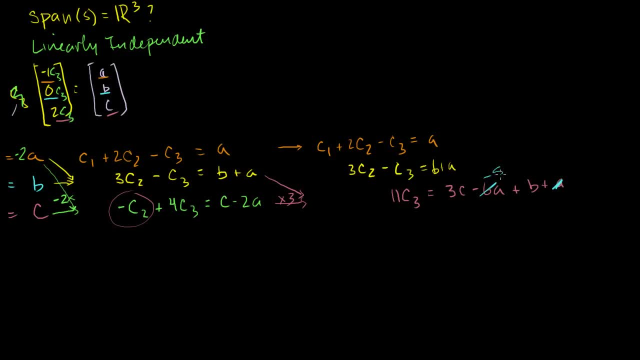 So let's just add them. So let's consider that a, and then this becomes minus 5a. So we get: and then if we divide both sides of this equation by 11, what do we get? We get: c3 is equal to 1 over 11 times 3c minus 5a. 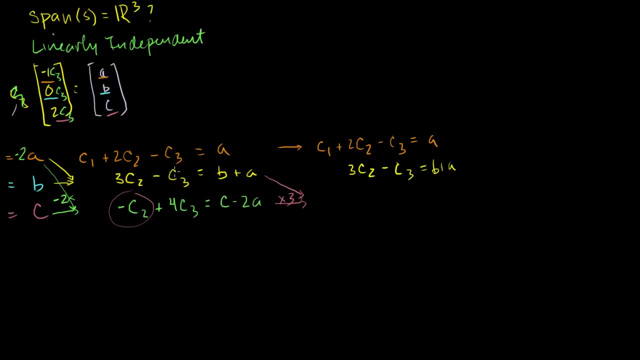 And then, when I multiply 3 times this, I get 12c3 minus a c3.. So that's 11c3.. And I multiply this times 3 plus this, So I get 3c minus 6a. I'm just multiplying this times 3 plus this. 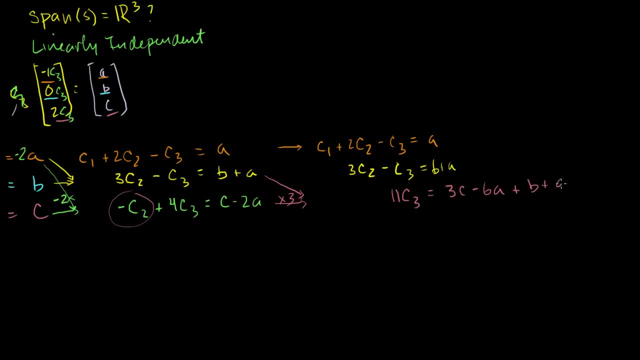 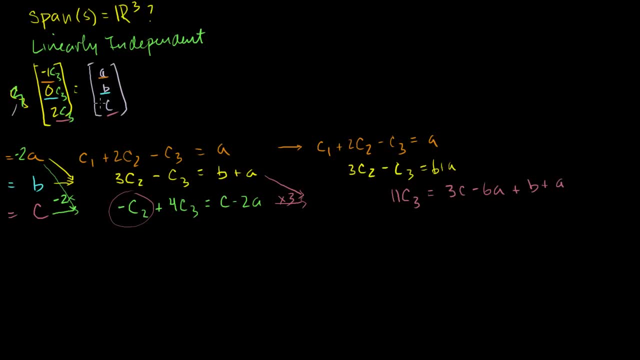 here and I think you realize that. But I just realized that I used the letter c twice and I just didn't want any confusion here. So this c that doesn't have any subscript is a different constant than all of these things over here. 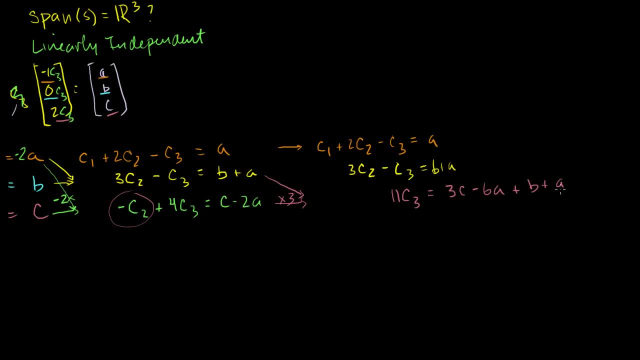 So let's see if we can simplify this. So we have an a and a minus 6a, So let's just add them. So let's consider that a, and then this becomes minus 5a, So we get, And then if we divide both sides of this equation by 11,. 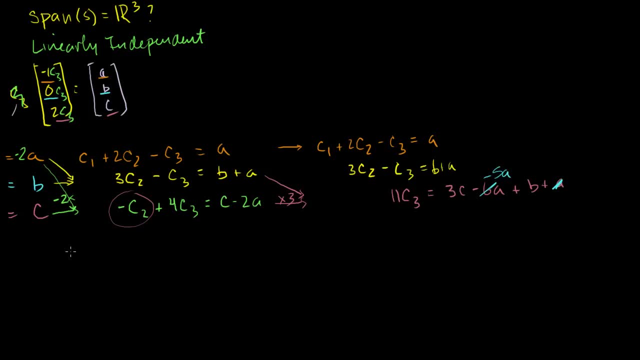 what do we get? We get: c3 is equal to 1 over 11 times 3c minus 5a. So you give me any a or c and I'll already tell you what c3 is. Now, what is c2?? 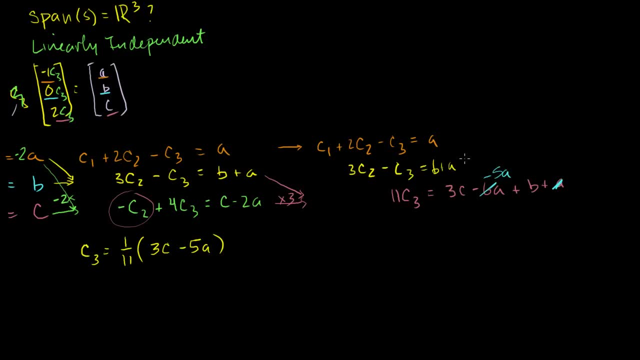 c2 is equal to. let me simplify this equation right here, Let me. Let me do it right there. So if I just add c3 to both sides of this equation, I get 3c2 is equal to b plus a plus c3.. 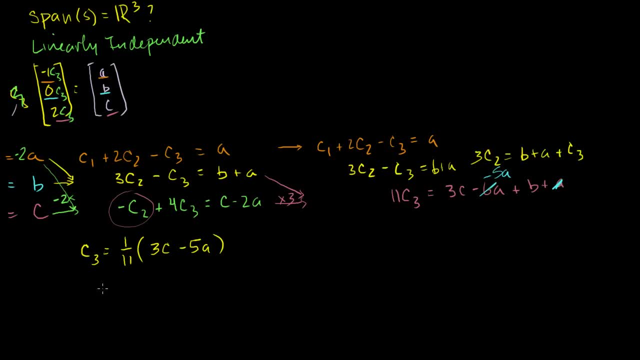 Well, I know, And if I divide both sides of this by 3, I get: c2 is equal to 1 over 3 times b plus a plus c3.. I'll just leave it like that for now. And then what is c1 is equal to? 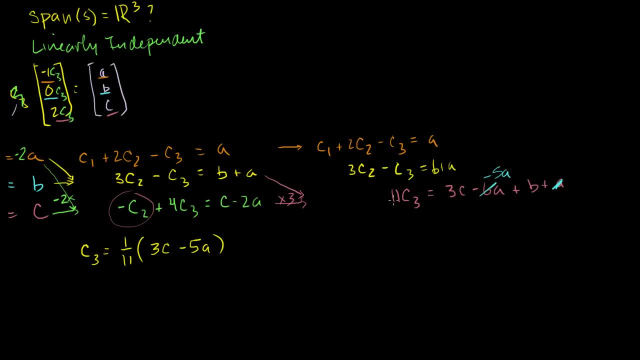 So you give me any a or c and I'll already tell you what c3 is. Now, what is c2?? c2 is equal to. let me simplify this equation right here. Let me do it right there. So if I just add c3 to both sides of the equation, 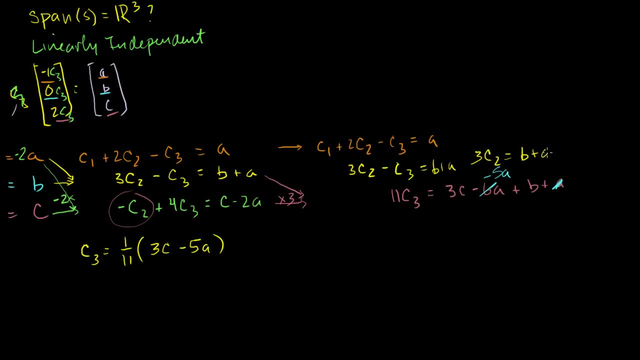 I get 3c2 is equal to b plus a plus c3.. And if I divide both sides of this by 3, I get c2 is equal to 1 over 3 times b plus a plus c3.. I'll just leave it like that for now. 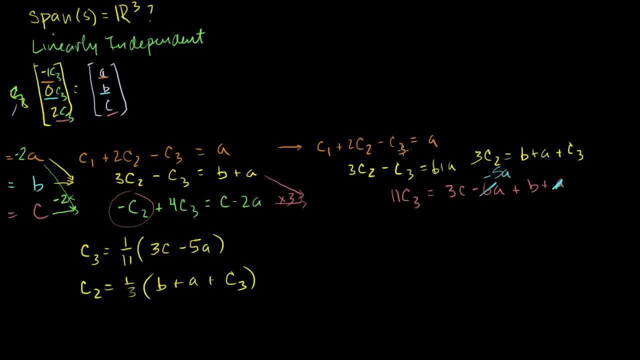 And then what is c1 is equal to? Well, If I could just rewrite this top equation as if I subtract 2c2 and add c3 to both sides, I get: c1 is equal to a minus 2c2 plus c3.. 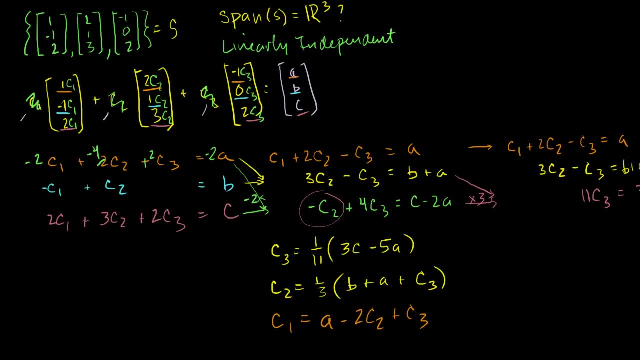 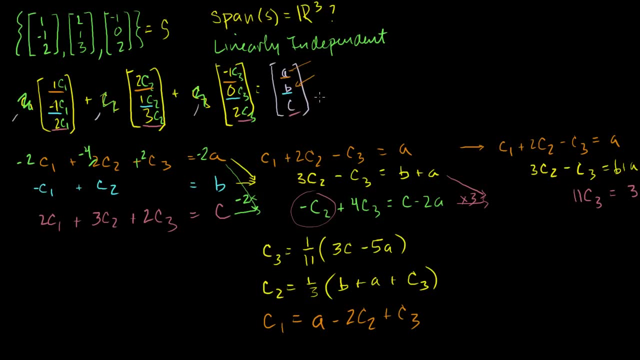 So what have I just shown you? You can give me any vector in R3 that you want to find. So you can give me any real number for a, any real number for b, Any real number for c, And if you give me those numbers, I'm claiming now that 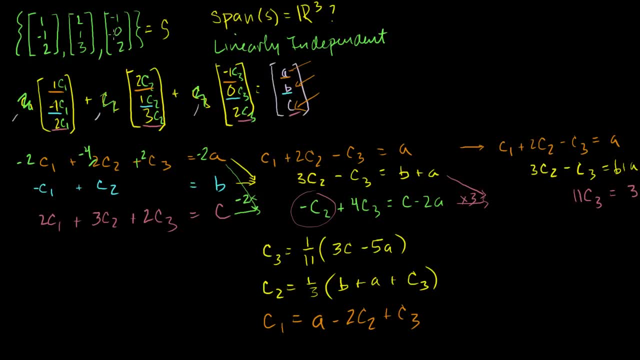 I can always tell you some combination of these three vectors that will add up to those, And I've actually already solved for what I have: to multiply each of those vectors by to add up to this third vector. So you give me your a's, b's and c's. 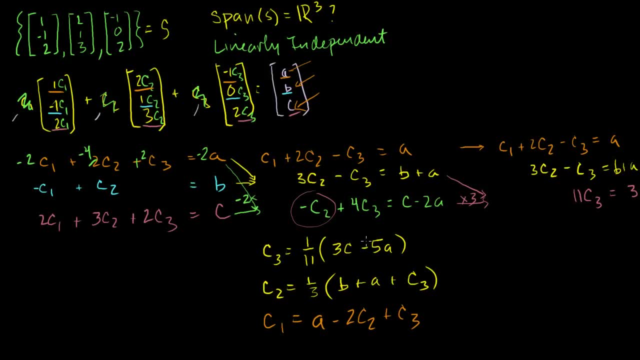 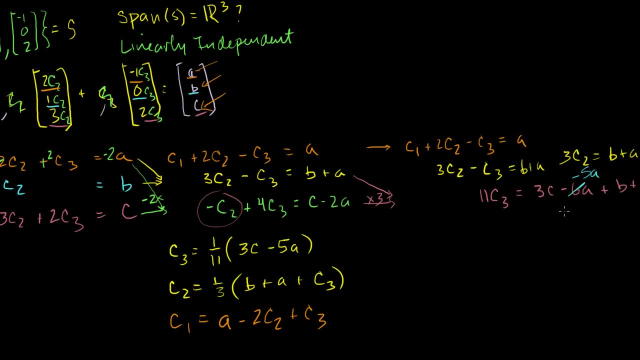 I just have to substitute into the a's and the c's right here. Oh sorry, I forgot this b over here. There's also a b. It was suspicious that I didn't have to do that. I have to deal with the b. 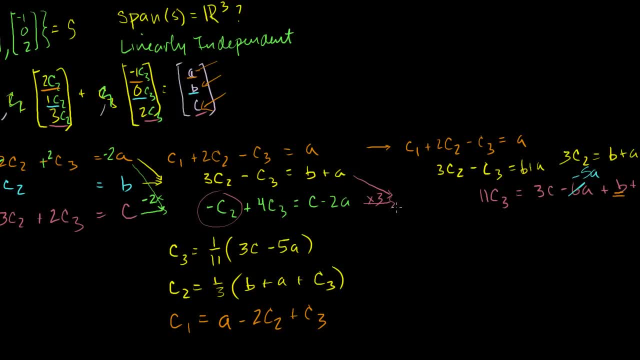 So there was a b right there. So this is 3c minus 5a plus b. Let me write that Plus a, b. There's a b right there in a parentheses, But I think you get the general idea. You give me your a's, b's and c's. 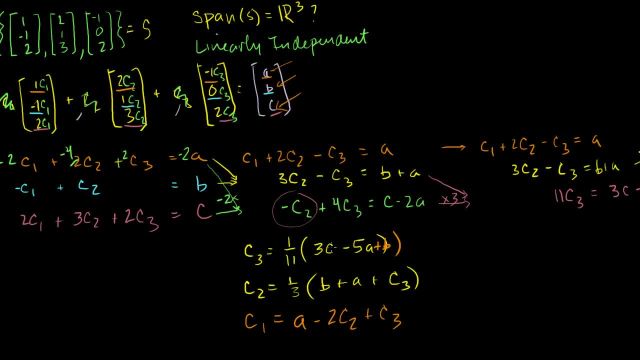 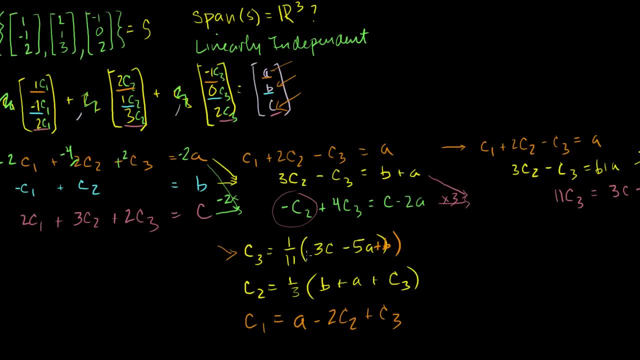 I'm going to give you a c3.. Now you gave me your a's, b's and c's. I got a c3.. This is just going to be another real number And I'm just going to take that with your former a's and. 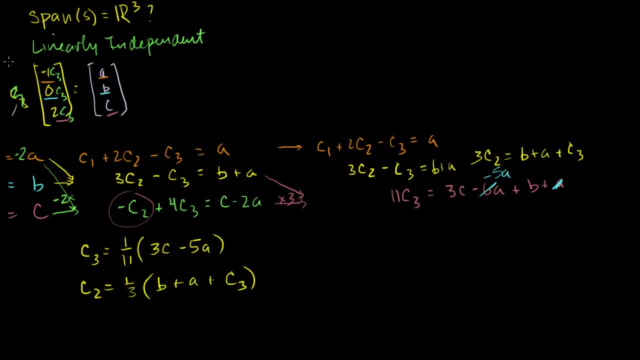 Well, if I I could just rewrite this top equation as: if I subtract 2c2 and add c3 to both sides, I get: c1 is equal to a minus 2c2 plus c3.. So what have I just shown you? 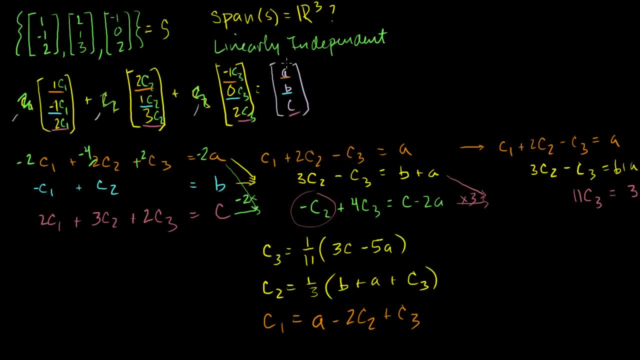 You can give me any vector in R3 that you want to find. So you can give me any real number for a, any real number for b, any real number for c, And if you give me those numbers, I'm claiming now that I 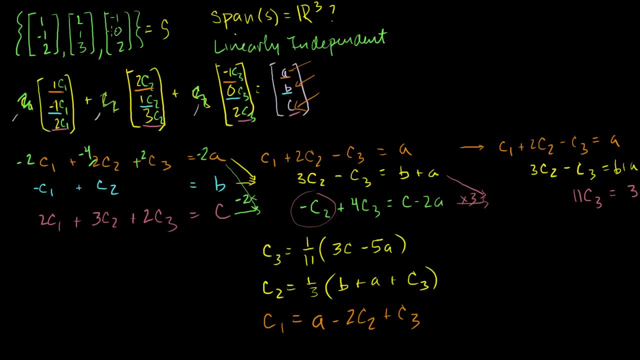 can always tell you some combination of these three vectors that will add up to those. And I've actually already solved for what I have: to multiply each of those vectors by to add up to this third vector. So you give me your a's, b's and c's. 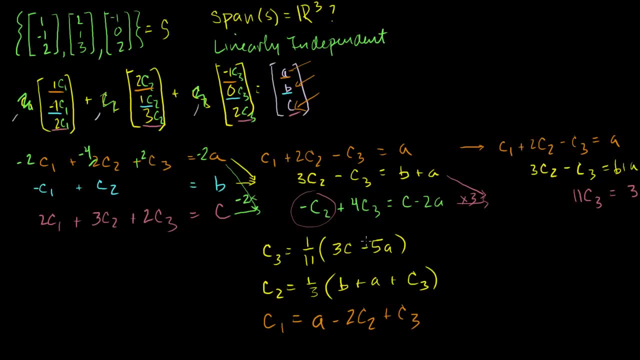 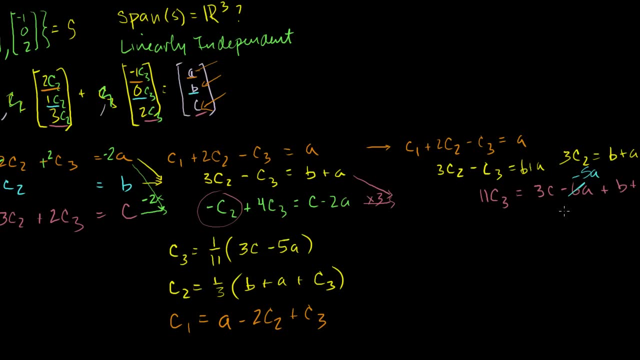 I just have to substitute into the a's and the c's right here. Oh sorry, I forgot this b over here. There's also a b. It was suspicious that I didn't have to deal with the b, so this is a. 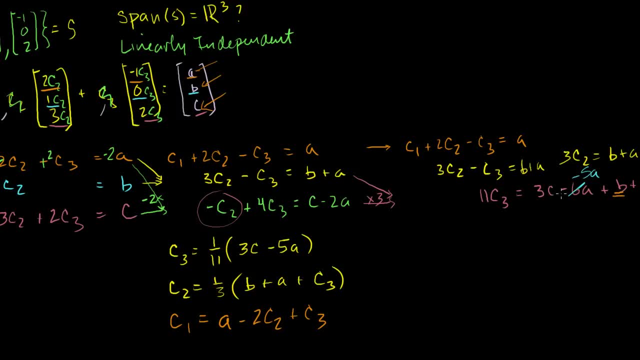 There was a b right there. So this is 3c minus 5a plus b. Let me write that Plus a b. There's a b right there in a parentheses, But I think you get the general idea. You give me your a's, b's and c's. 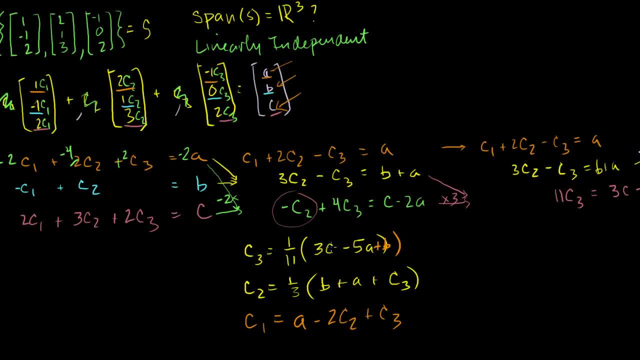 Any real numbers can apply. I'm not dividing by. There's no division over here, so I don't have to worry about dividing by 0.. So this is just a linear combination of any real numbers. so I can clearly get another real number. 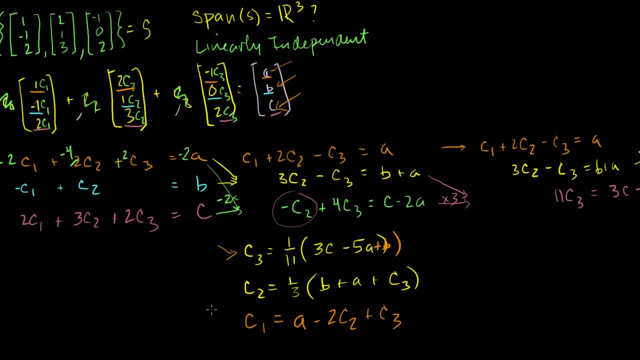 So you give me your a's, b's and c's, I'm going to give you a c3.. Now you gave me your a's, b's and c's, I got a c3.. This is just going to be another real number. 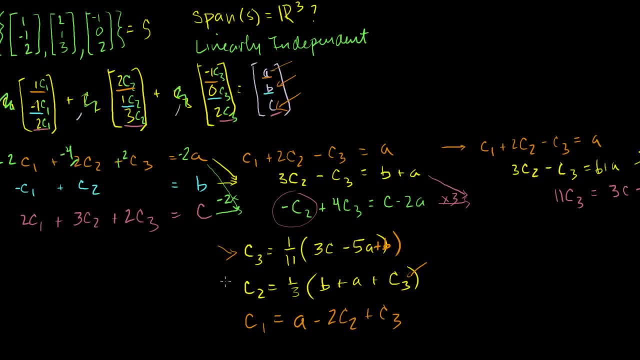 And I'm just going to take that with your former a's and b's and I'm going to be able to give you a c2.. And then we're already able to solve for a c2 and a c3. And then I just use your a as well. 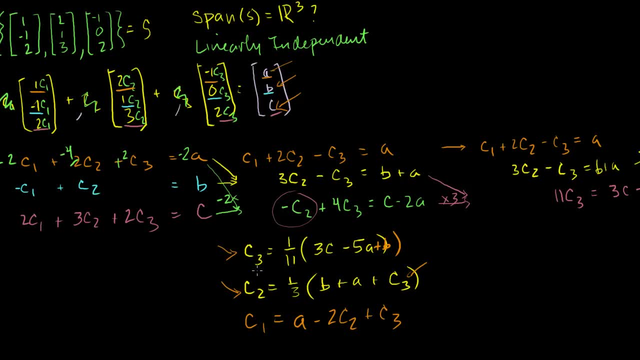 b's and I'm going to be able to give you a c2.. And then we're already able to solve for a c2 and a c3.. And then I just use your a as well, And then I'm going to give you a c1. 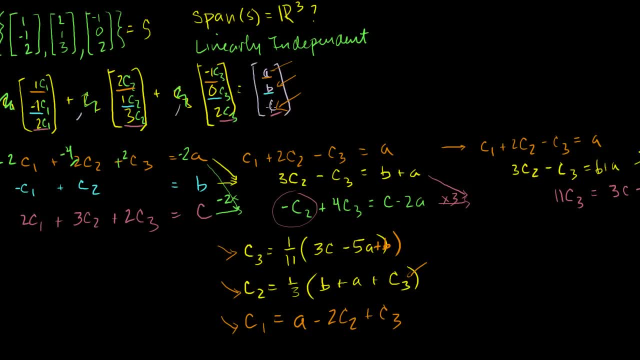 So hopefully you're seeing that no matter what a, b and c you give me, I can give you a c1,, c2, or c3.. There's no reason that any a's, b's or c's should break down these formulas. 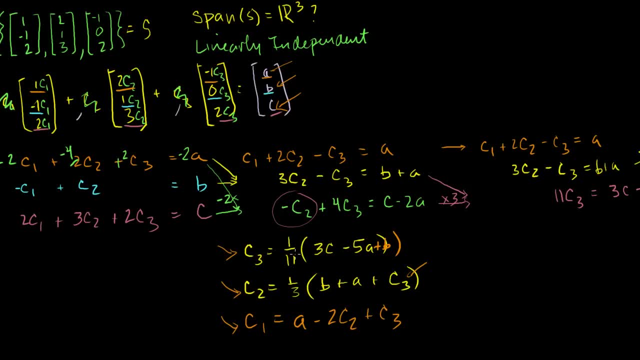 We're not doing any division, so it's not like a 0 would break it down. So I can say definitively that the set of vectors, of these three vectors, does indeed span R3.. Now let me ask you another question, where I already 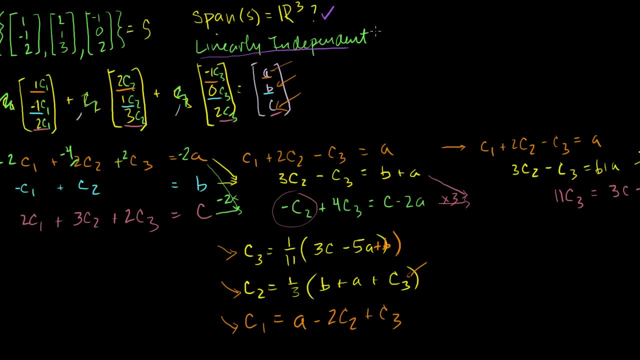 asked it: Are these vectors linearly independent? Now, we said that, in order for them to be linearly independent, the only solution, the only solution to c1 times my first vector, 1 minus 1, 2, plus c2 times my second vector, 2, 1, 3, plus c3. 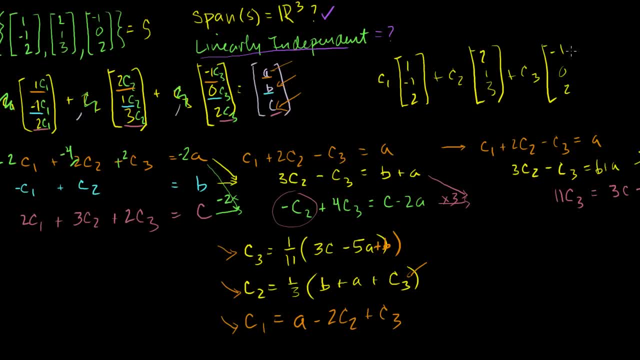 times my third vector minus 1, 0, 2.. So if something is linearly independent, that means that the only solution to this equation- so if I take any common- there's the only solution to this equation. so if I want to find some set of combinations of these vectors, 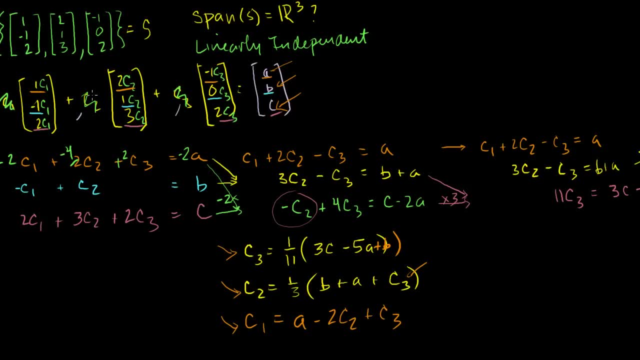 And then I'm going to give you a c1.. So hopefully you're seeing that no matter what a, b and c you give me, I can give you a c1, c2, or c3. There's no reason that any a, b and c can't be a c1, c2, or c3.. 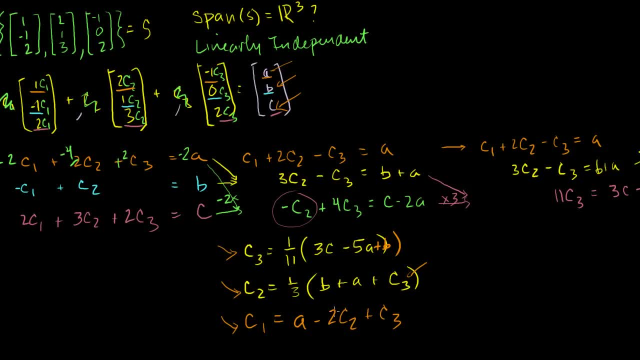 There's no reason that any a, b and c can't be a, c1,, c2, or c3.. There's no reason that any a, b and c3 should break down these formulas. We're not doing any division, so it's not like a 0 would. 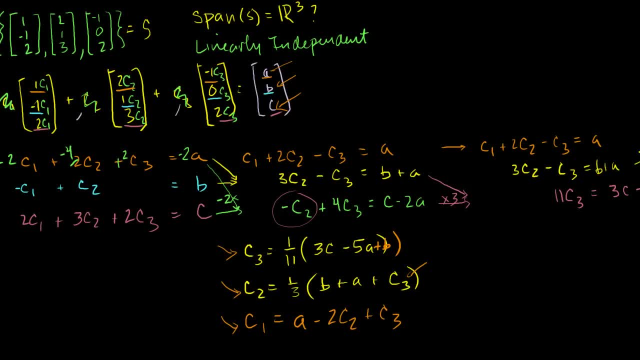 break it down. So I can say definitively that the set of vectors, of these three vectors, does indeed span R3.. Now let me ask you another question, where I already asked it: Are these vectors linearly independent? Now, we said that in order for them to be linearly. 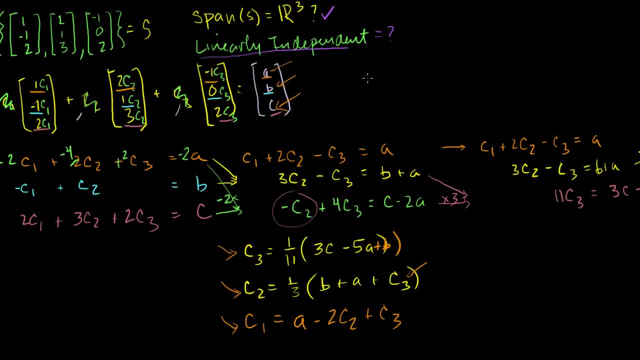 independent. the only solution to c1 times my first vector 1 minus 1,, 2, plus c2 times my second vector 2, 1,, 3, plus c3 times my third vector minus 1,. 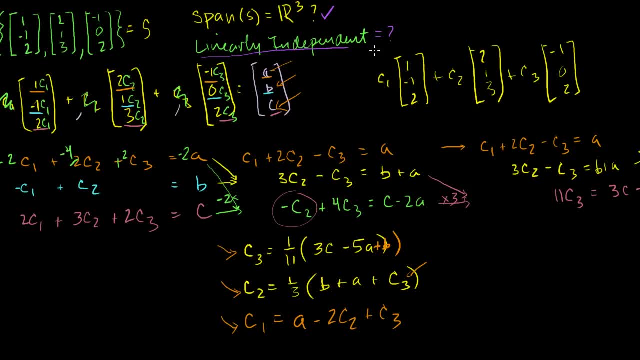 0, 2.. So if something is linearly independent, that means that the only solution to this equation- so if I take any common, there's the only solution to this equation. So if I want to find some set of combinations of these vectors that add up to 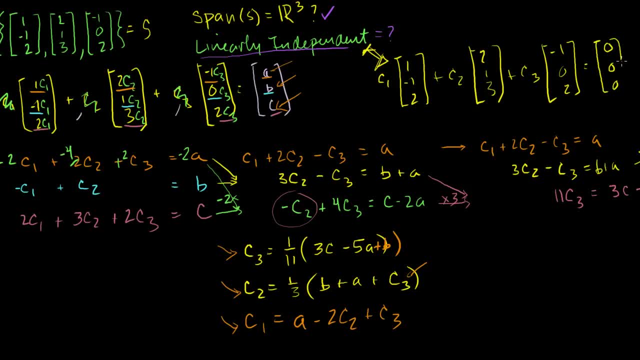 the zero vector, and I did that in the previous video. if they are linearly dependent, there must be some non-zero solution. So one of these constants, at least one of these constants, would be non-zero for this solution. I mean, you can always make them 0,, no matter what. but if 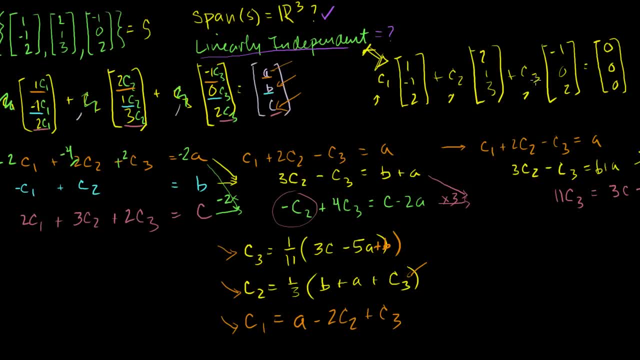 they're linearly dependent, then one of these could be non-zero. If they're linearly independent, they're linearly independent, Yeah, Then all of these have to be. the only solution to this equation would be c1, c2, c3: all have to be equal to 0. 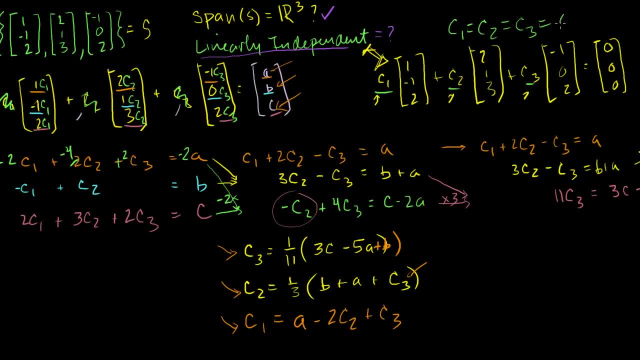 c1,, c2, c3 all have to be equal to 0. Linear independence implies this. This implies linear independence. Now, this is the exact same thing we did here, but in this case I'm just picking my a, b's and c's to be 0. 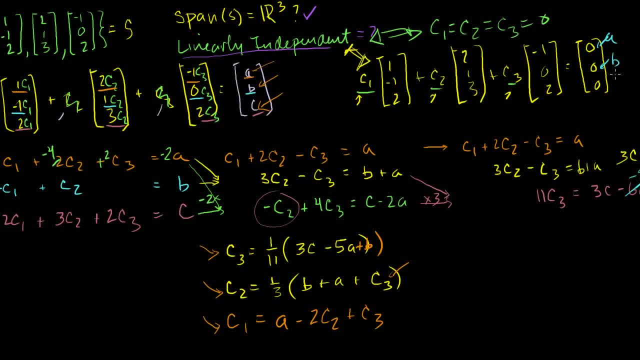 This is a, this is b and this is c. right, I can pick any vector in R3 for my a's, b's and z's. I'm now picking the 0 vector, So let's see what our c1, c2's and c3's are. 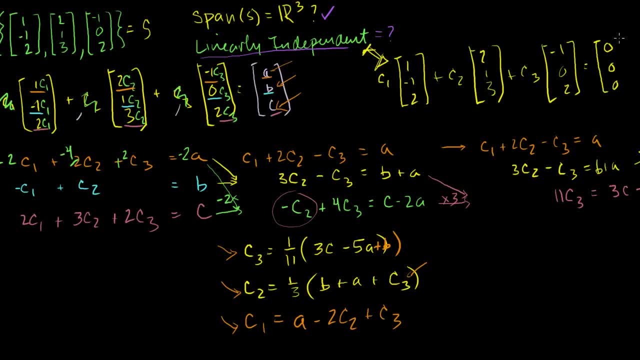 that add up to the zero vector, and I did that in the previous video. if they are linearly dependent, there must be some non-zero solution. So at least one of these constants would be non-zero for this solution. I mean, you can always make them 0,, no matter what. but if 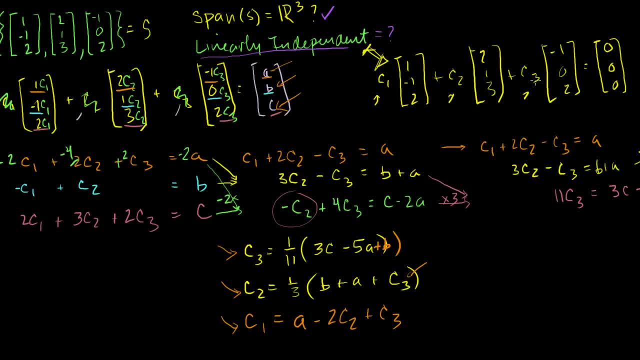 they're linearly dependent, then one of these could be non-zero. If they're linearly independent, so one of the independent, then all of these have to be. the only solution to this equation would be c1, c2, c3. all have to be equal to. 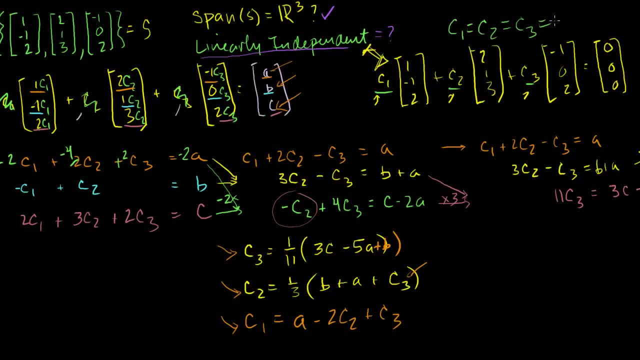 0.. c1,, c2, c3 all have to be equal to 0.. Linear independence implies this. This implies linear independence. Now, this is the exact same thing we did here, but in this case I'm just picking my a, b's and c's to be 0.. 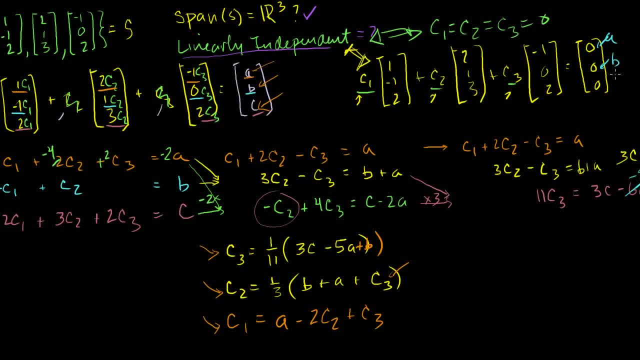 This is a, this is b and this is c. I can pick any vector in R3 for my a's, b's and z's. I'm now picking the 0 vector, So let's see what our c1, c2's and c3's are. 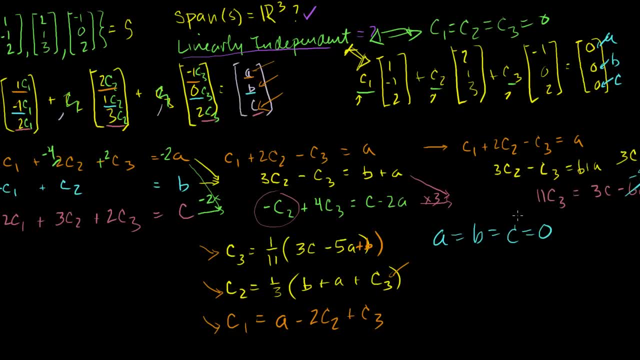 So my a equals b is equal to c is equal to 0.. I'm setting it equal to the 0 vector. What linear combination of these three vectors equal the 0 vector? Well, if a, b and c are all equal to 0.. 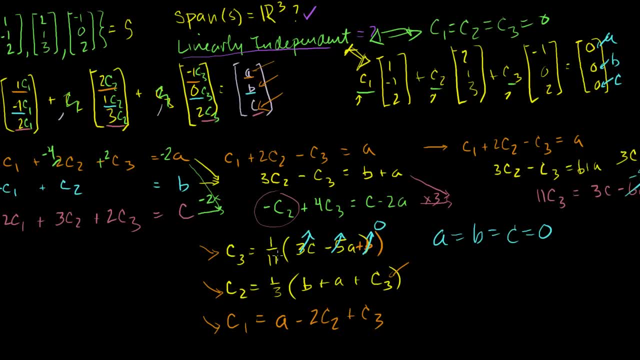 That term is 0. That is 0. That is 0. You have 1, 11th times 0 minus 0 plus 0. That's just 0. So c3 is equal to 0.. Now, c3 is equal to 0.. 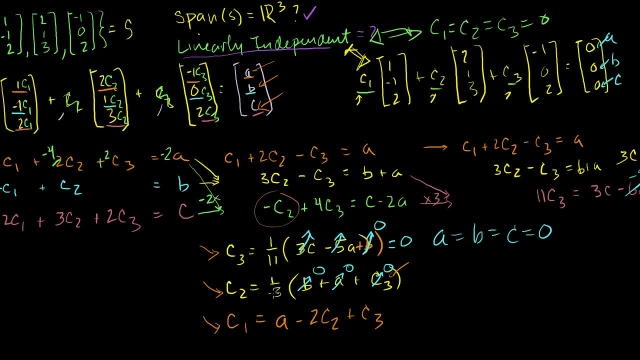 We already know that a is equal to 0 and b is equal to 0.. c2 is 1, third times 0. So it equals 0.. Now, what's c1?? Well, it's c3, which is 0.. 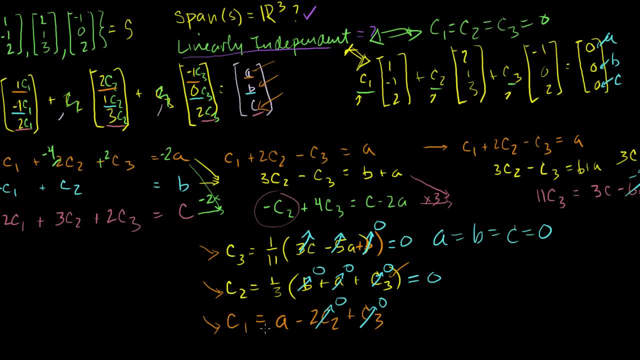 c2 is 0. So 2 times 0 is 0. So c1 is just going to be equal to a. What I just said, a is equal to 0.. So the only solution to this equation right here, the only linear combination of these three vectors, that 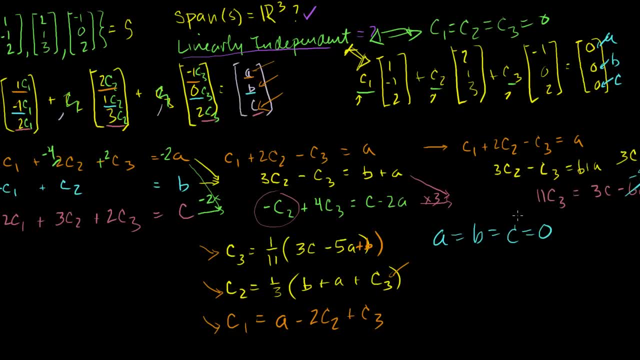 So my a equals b is equal to c is equal to 0.. I'm setting it equal to the 0 vector. What linear combination of these three vectors equal the 0 vector? Well, if a, b and c are all equal to 0.. 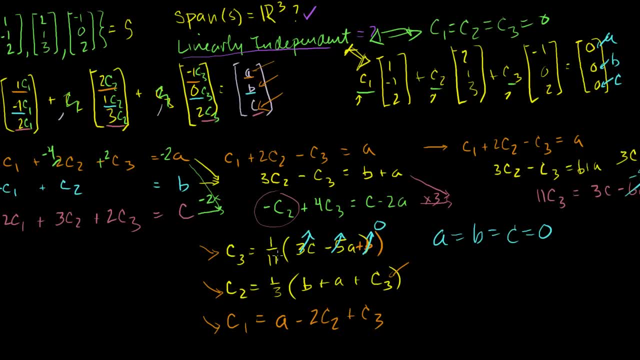 That term is 0. That is 0. That is 0. You have 1, 11th times 0 minus 0 plus 0. That's just 0. So c3 is equal to 0.. Now, c3 is equal to 0.. 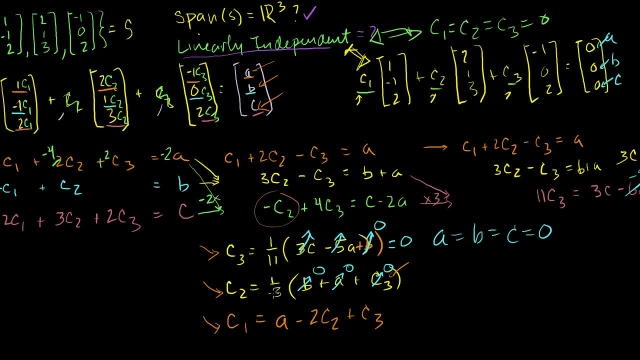 We already know that a is equal to 0 and b is equal to 0.. c2 is 1, third times 0. So it equals 0.. Now, what's c1?? Well, it's c3, which is 0.. 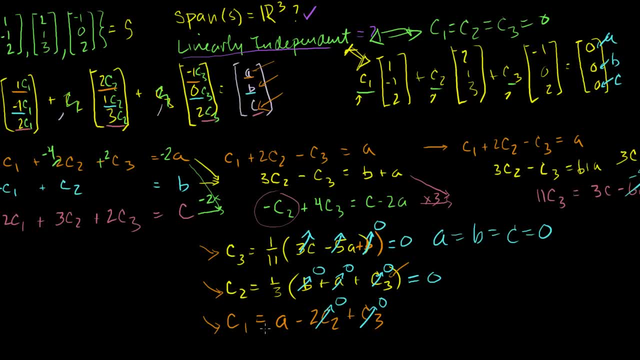 c2 is 0. So 2 times 0 is 0. So c1 is just going to be equal to a. What I just said, a is equal to 0.. c2 is equal to 0.. So the only solution to this equation, right here: 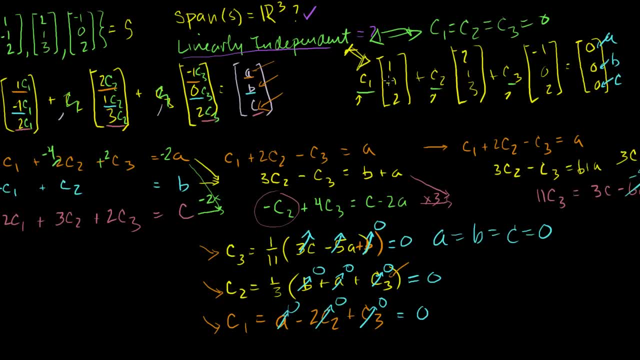 the only linear combination of these three vectors that result in the 0 vector are when you weight all of them by 0. So I just showed you that c1, c2, and c3 all have to be 0. And because they're all 0, we know. 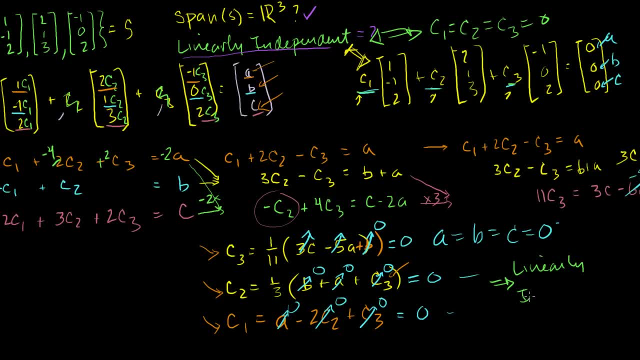 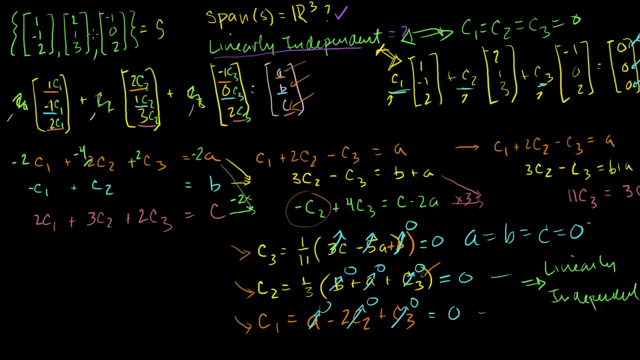 that this is a linearly independent equation, It's a linearly independent set of vectors, Or that none of these vectors can be represented as a combination of the other two. None of these vectors can be represented as a combination of another two. So this is interesting. 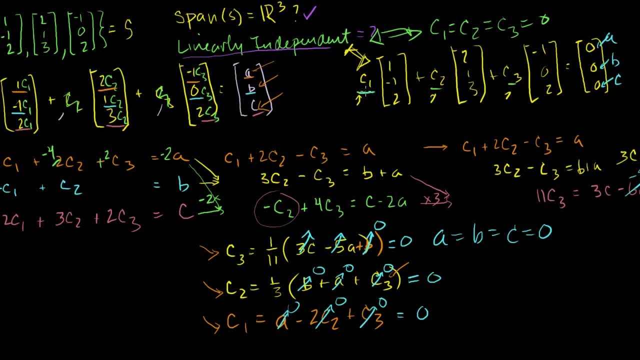 result in the 0 vector are when you weight all of them by 0. So I just showed you that c1, c2, and c3 all have to be 0. And because they're all 0, we know that this is a linearly. 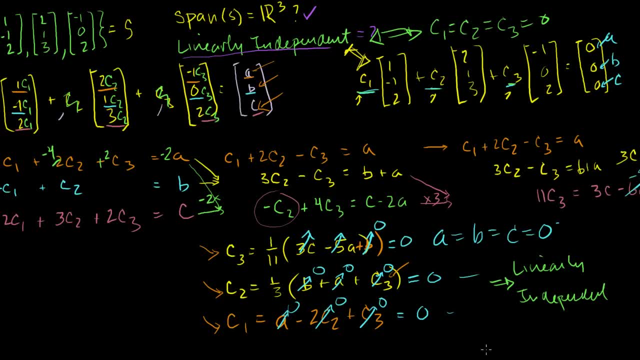 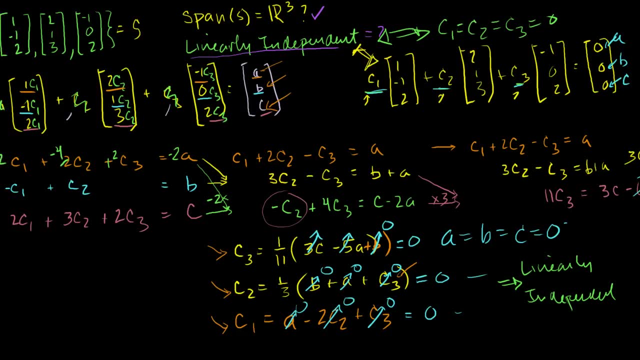 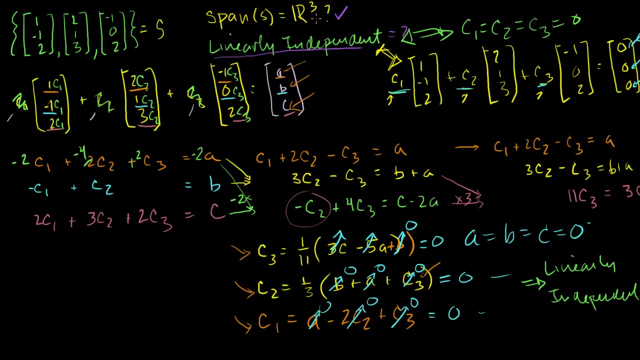 independent equation, It's a linearly independent set of vectors, Or that none of these vectors can be represented as a combination of the other two. None of these vectors can be represented as a combination of another two. So this is interesting. I have exactly three vectors that span r3, and they're 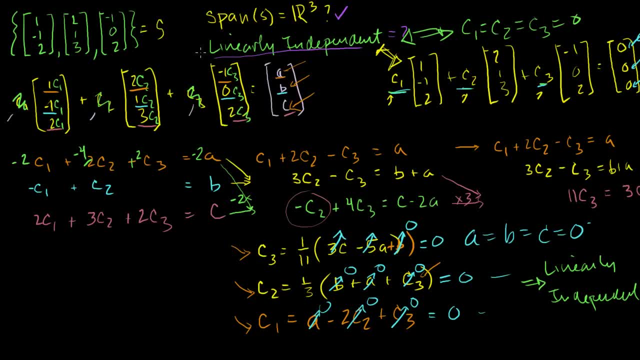 linearly independent And linearly independent. in my brain that means that, look, I don't have any redundant vectors, anything that could have just been built with the other vectors, And I have exactly three vectors And it's spanning r3.. 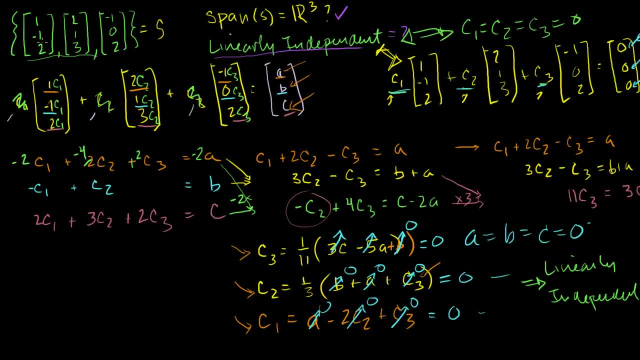 So in general- and I haven't proven this to you, but I could- is that if you have exactly three vectors and they do span r3, they have to be linearly independent. If they weren't linearly independent, then one of 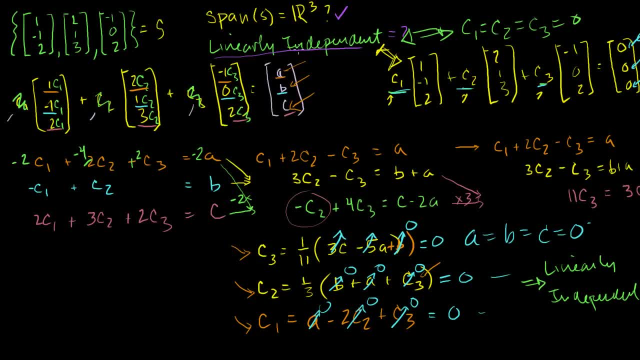 I have exactly three vectors that span r3, and they're linearly independent, And linearly independent in my brain that means that, look, I don't have any redundant vectors, anything that could have just been built with the other vectors. 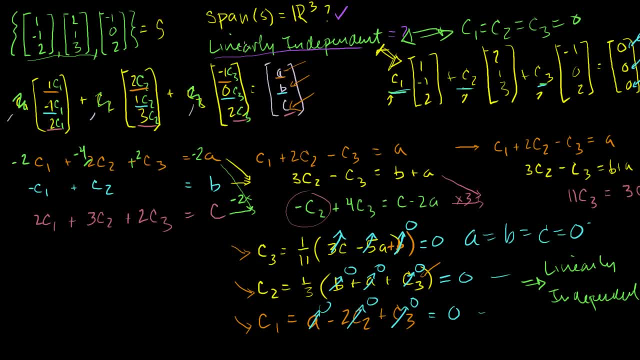 And I have exactly three vectors And it's spanning r3.. So in general- and I haven't proven this to you but I could- is that if you have exactly three vectors and they do span r3, they have to be linearly independent. 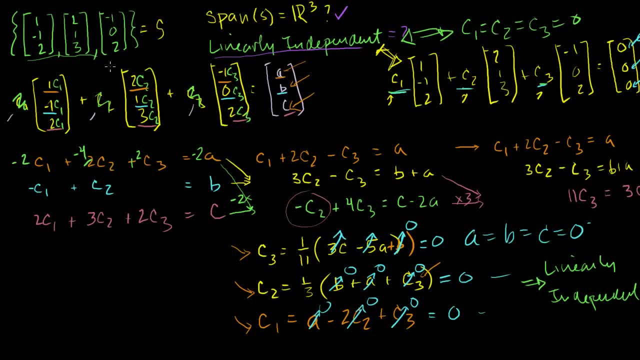 If they weren't linearly independent, then one of these would be redundant. Then you know, let's say that that guy was a redundant one. I always pick the third one. But let's say this guy would be redundant, which means that 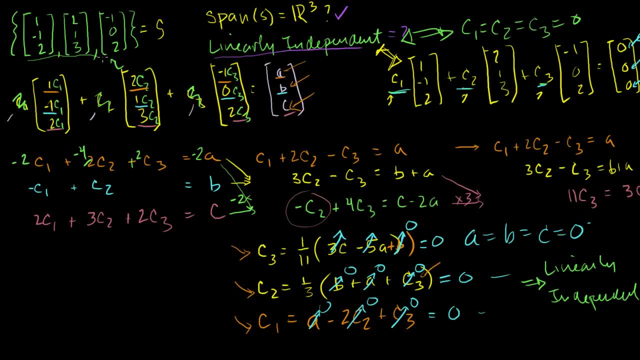 these would be redundant. Then you know, let's say that that guy was a redundant one. I always pick the third one. But let's say this guy would be redundant, which means that the span of this would be equal to the span of these two. 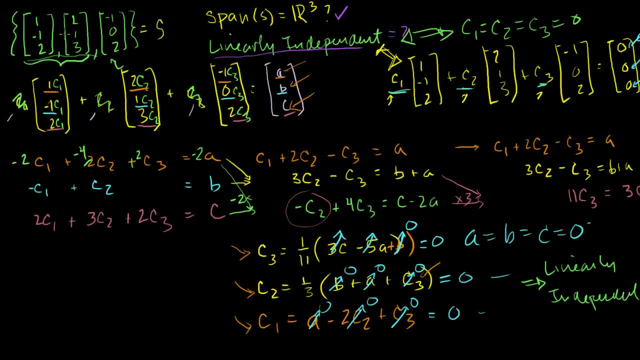 right, because if this guy is redundant he could be part of the span of these two. Right, These two guys And the span of two vectors could never span r3.. Or in the other way you could go if you have three linear. 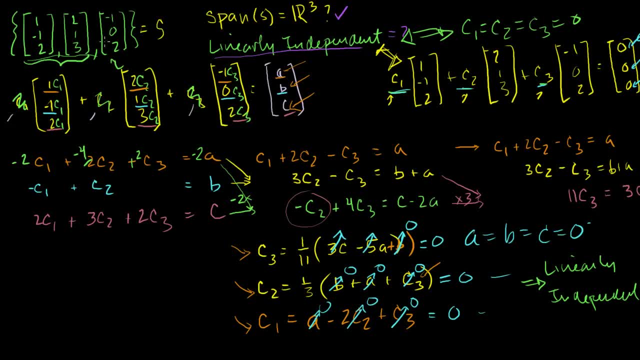 independent. three tuples and they're all independent. then you could also say that that spans r3.. But I haven't proven that to you. but hopefully you get the sense that, look, each of these is contributing new directionality right. 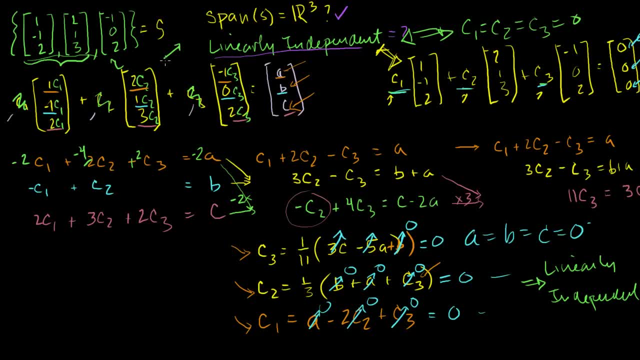 One is, you know, going like that. They might they're not completely orthogonal to each other, but they're giving just enough directionality that you can kind of add a new dimension To what's going on. So hopefully that helped you a bit and I'll see you in the next video. 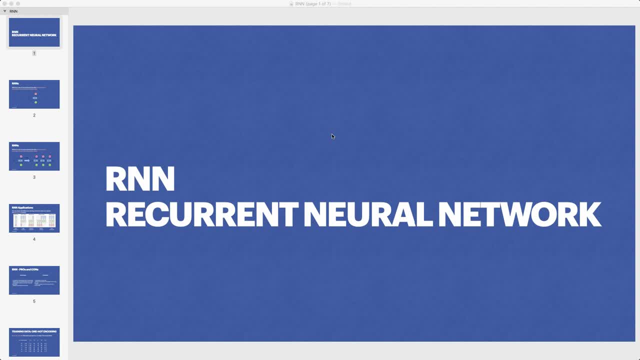 Hey guys, welcome to a new PyTorch tutorial. Today we'll be talking about recurrent neural nets, or short RNNs. I will briefly explain the theory behind RNNs and the different kind of applications, And then we will implement a RNN from scratch in PyTorch to do name classification. This should: 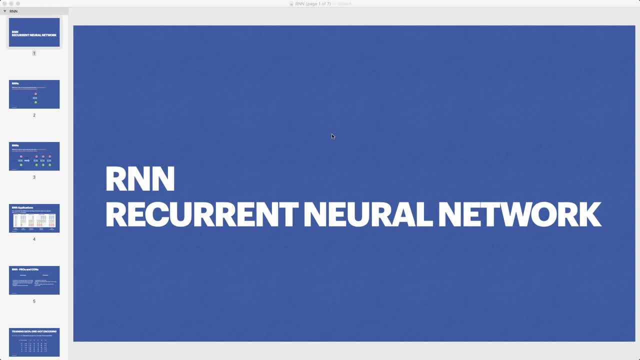 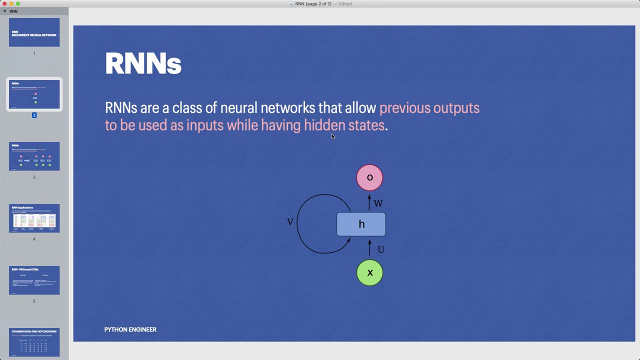 give you a good understanding of how RNNs work internally. So let's start. RNNs are a class of neural networks that allow previous outputs to be used as inputs, while having hidden states. Here's an image that shows the architecture of RNNs in the simplest way. So we have an input and 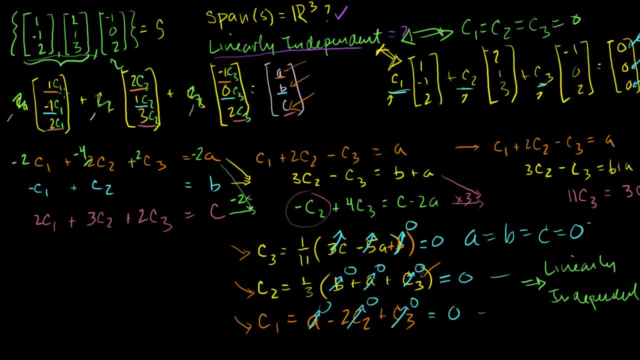 the span of this would be equal to the span of these two, Because if this guy is redundant he could be part of the span of r3. These two guys And the span of two vectors could never span r3. Or in the other way you could go if you have three linear. 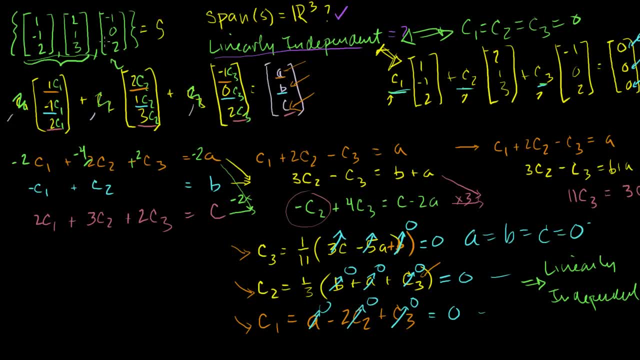 independent. three tuples and they're all independent. then you could also say that that spans r3.. But I haven't proven that to you. But hopefully you get the sense that, look, each of these is contributing new directionality right. 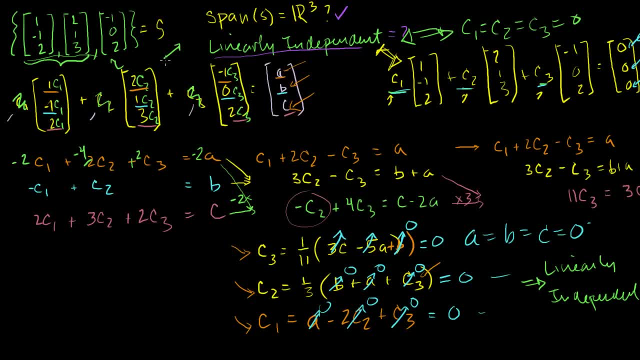 One is, you know, going like that. They're not completely orthogonal to each other, but they're giving just enough directionality that you can kind of add a new dimension To what's going on. So hopefully that helped you a bit and I'll see you in the next video. 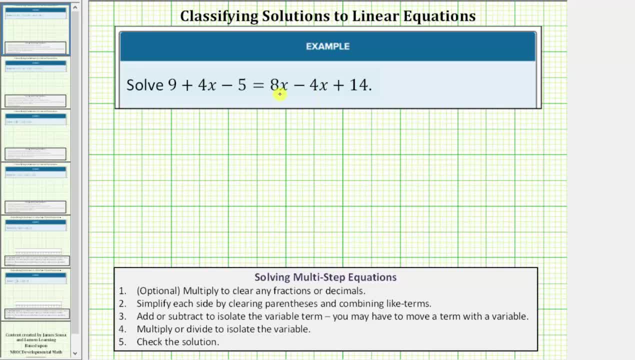 We want to solve the given linear equation. Normally, when solving a linear equation in one variable, we expect one solution, but that's not always the case. Let's attempt to solve this equation and see what happens, Following the guidelines to solve multi-step equations. 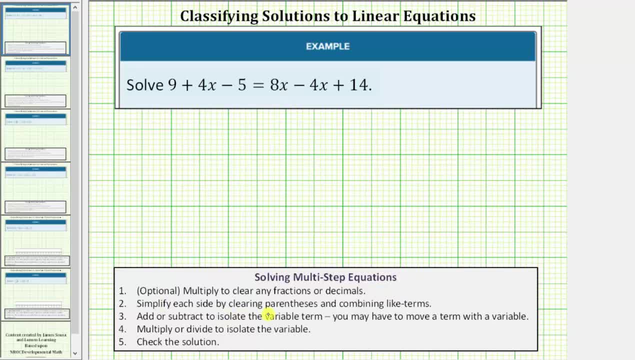 the first thing we do for this equation would be to simplify each side by clearing parentheses and combining like terms. Notice: on the left side we have two constant terms. On the right side we have two x terms. So on the left side, nine minus five is equal to four. 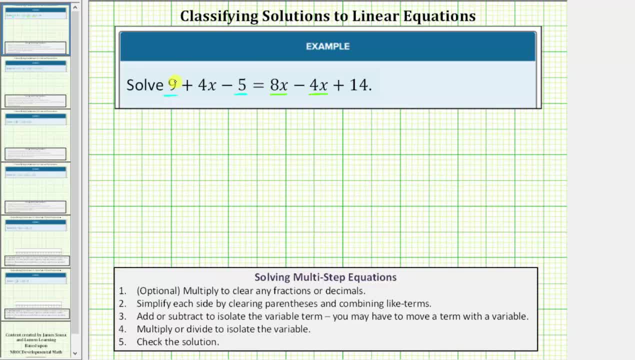 and therefore the left side simplifies to four plus four x or four x plus four. Now, on the right side, eight x minus four x is four x. The right side simplifies to four x plus 14.. The next step is to add or subtract.